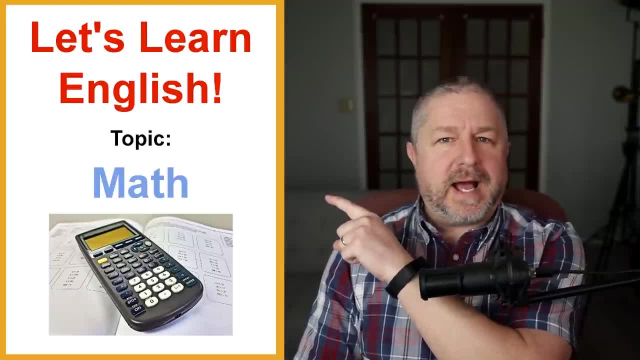 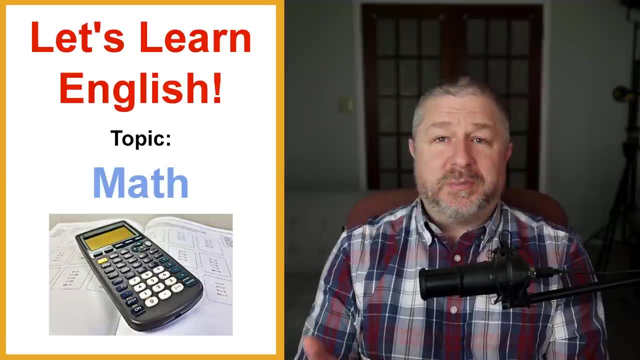 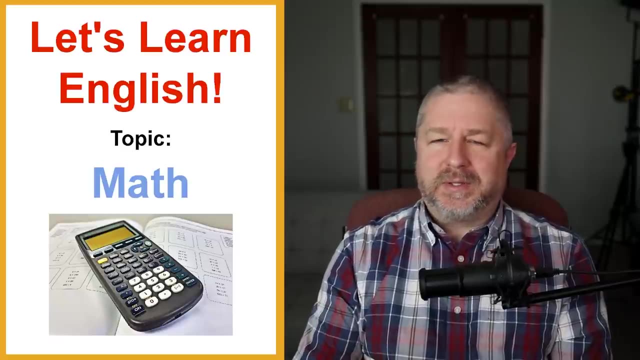 Well, hello and welcome to this English lesson about math. I'm not sure which subjects in school were your favorite. Maybe math class was an enjoyable place for you to be. Maybe math class was really, really boring. But either way, whether you like math or don't like math, I think this will be. 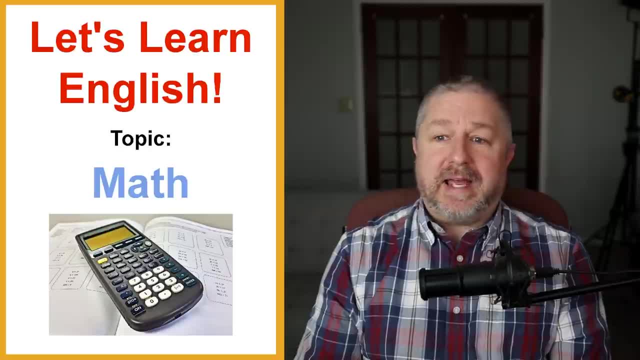 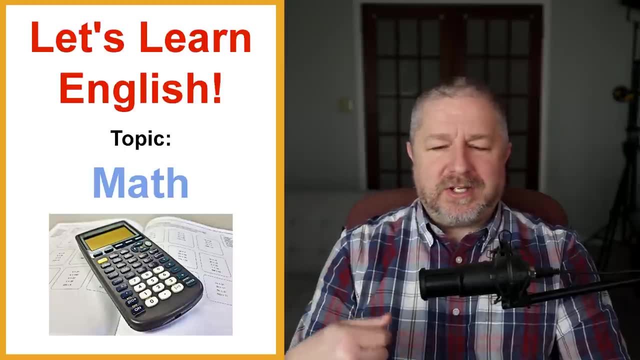 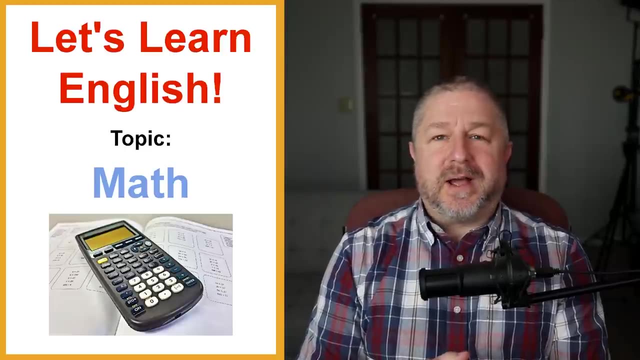 a good English lesson for you. We all use math every day somewhere, Whether it's figuring out how much money we need to pay for something and how much change we get, or just trying to calculate how much we have to buy if we're building something. We sometimes need to use math, and so in this English 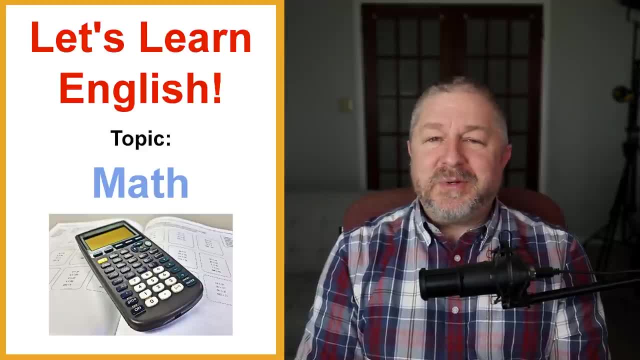 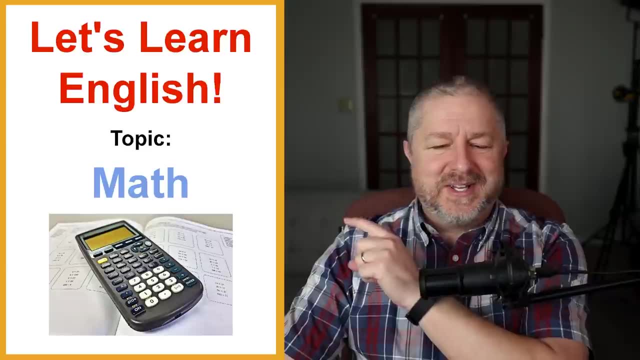 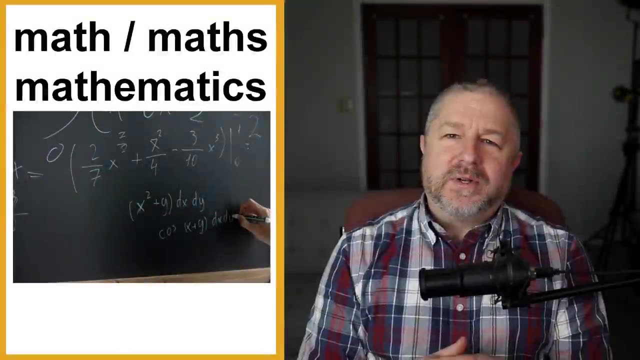 lesson. I'll talk a little bit about math. Um, I have to admit some of the slides. there's a lot less pictures in the slides and a lot more numbers in the slides. So, uh, once again, welcome to this English lesson about math. So you'll notice I 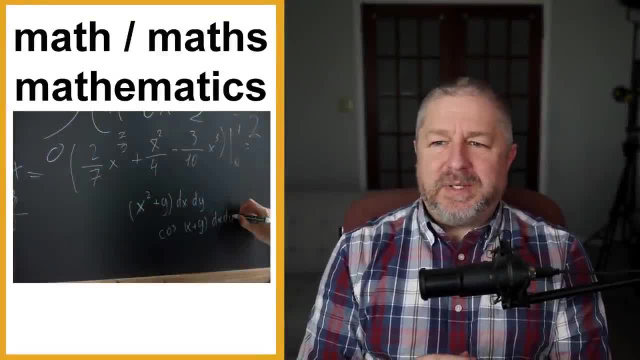 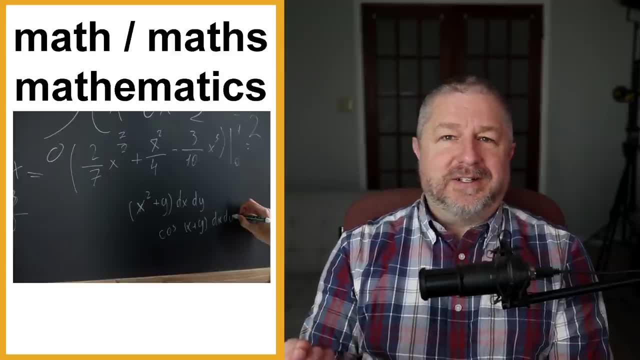 have the word math and I have the word maths here, and that's because there's a difference between North American English, where we use the short form math, and British English, where they often say maths. So for me I just say math When I 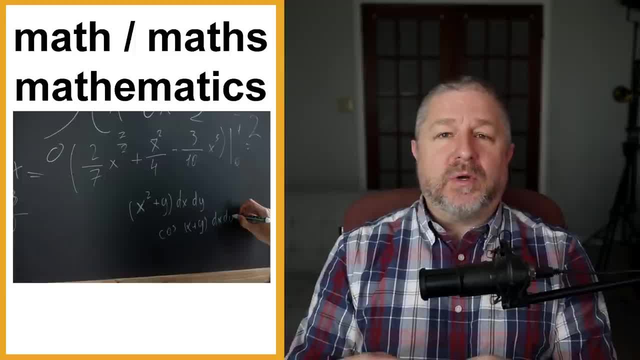 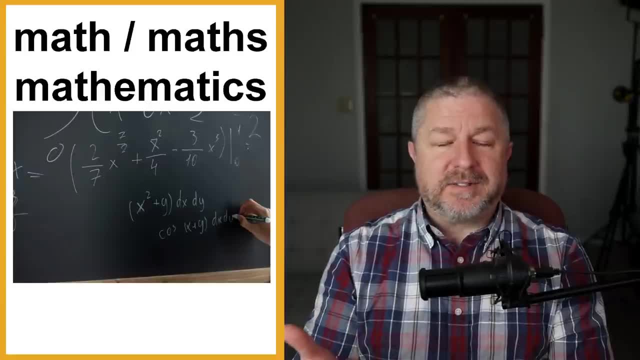 talk about numbers and adding and subtracting. when I talk about going to a class where I'm going to learn about mathematics, I would say math, I would just call it math class. So uh again, if you are on the other side of the 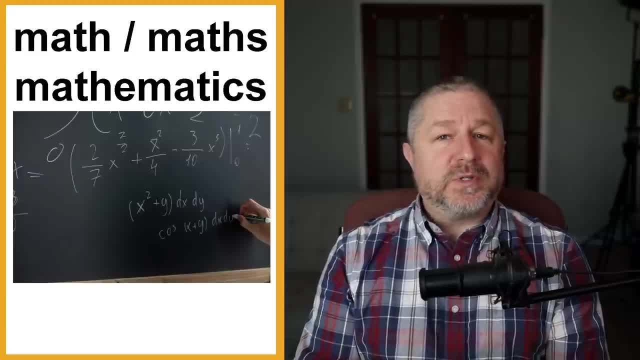 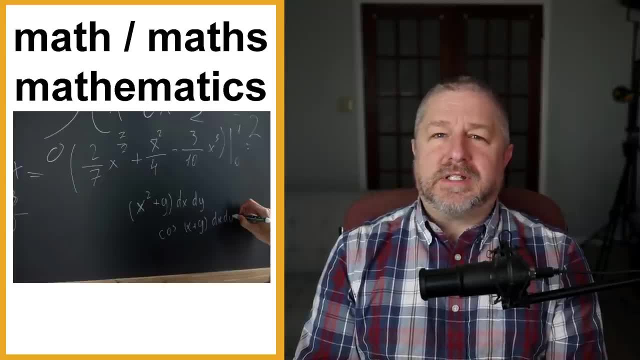 Atlantic. if you are learning British English, uh, you would most likely say maths, and both are more common than the word mathematics. We don't often say, um, I'm going to take a class on mathematics. We would instead say, I'm going to take. 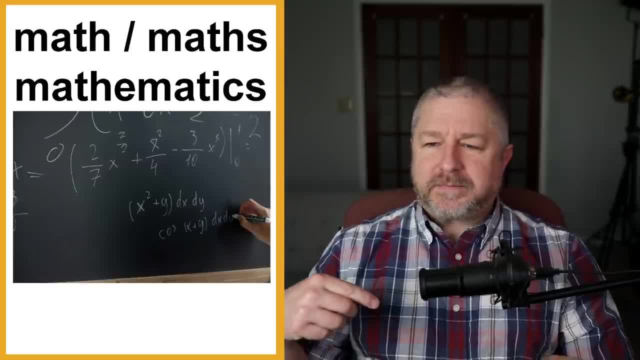 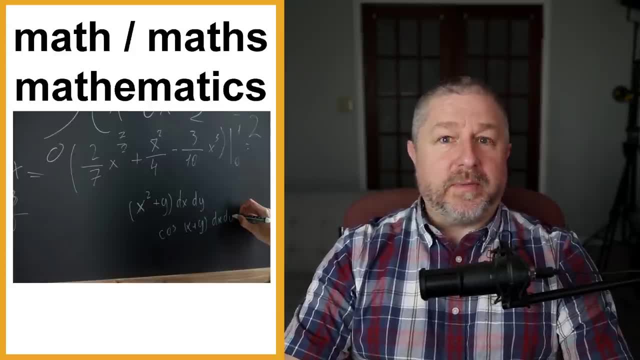 a math class. So mathematics, the study of, uh, numbers and equations, and all of that fun stuff which I will explain in a bit. Uh, math, the short form that I use, and maths, the short form that I use in mathematics. I use them in all of my classes. 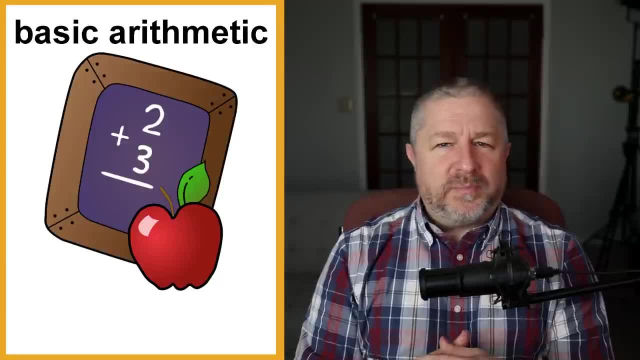 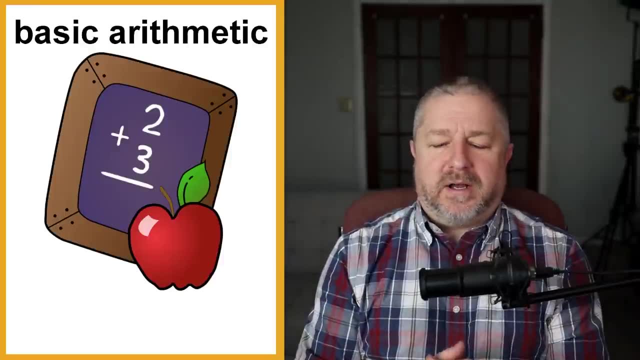 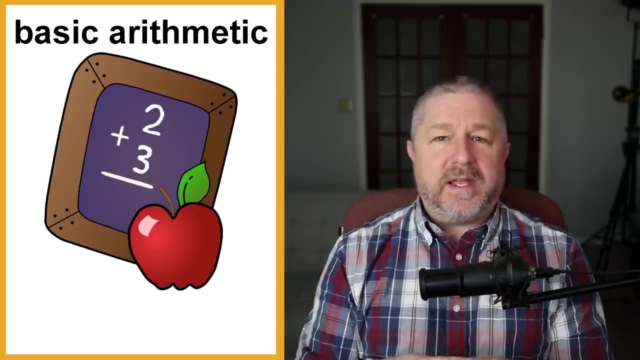 if they are over there in Britain across the way, We also have what's called basic arithmetic, So mathematics is a general term for everything to do with math, but when we talk about basic arithmetic we're talking about adding, subtracting, multiplying and dividing. Kids when they go to 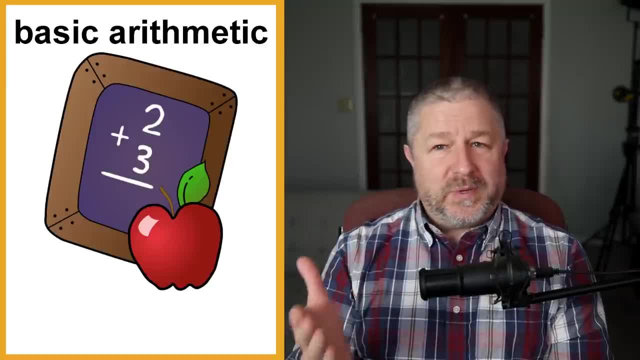 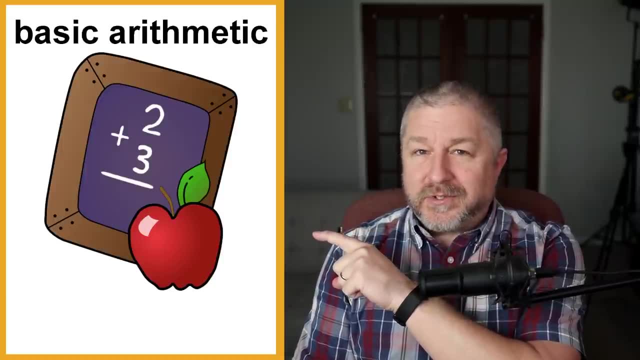 school, one of the first things they learn is basic arithmetic. They learn to read, They learn to write And they learn how to do basic arithmetic. So that's things like this, where you see two plus three, which equals five, by the way. So you're hearing me already. 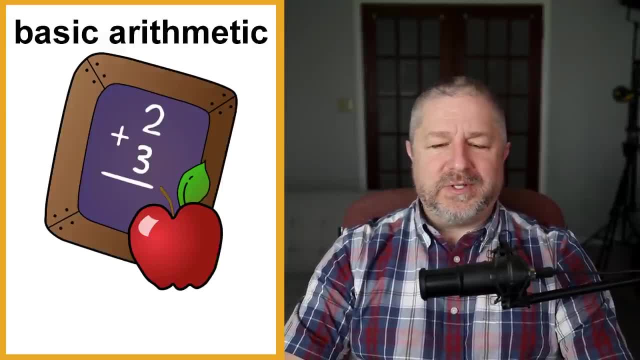 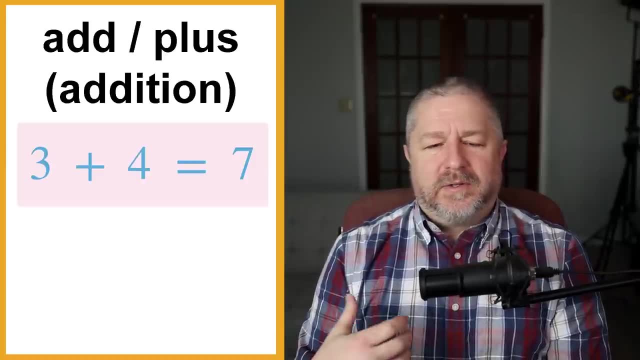 start to use some of the English language we would use when talking about math. So let's get to the four- uh, most common. So you'll notice I've put a number of words at the top because some of these are used to describe the equation. 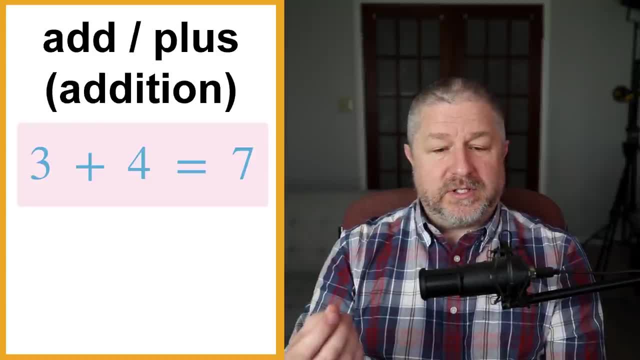 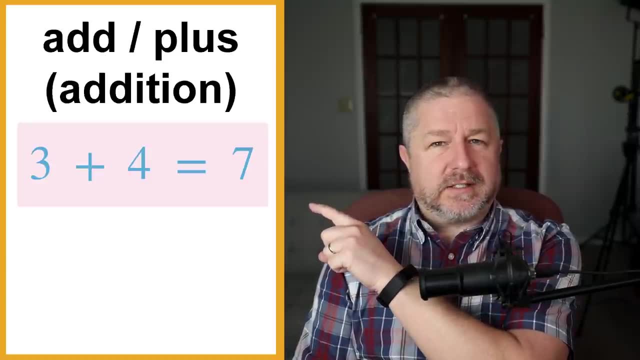 and some are used to refer to the equation. So when you add two numbers, you use the plus sign and you end up with an equation like this. So if I wanted to add three and four, I would say three plus four equals. 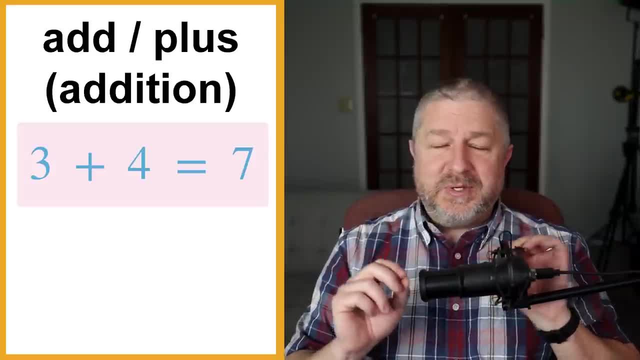 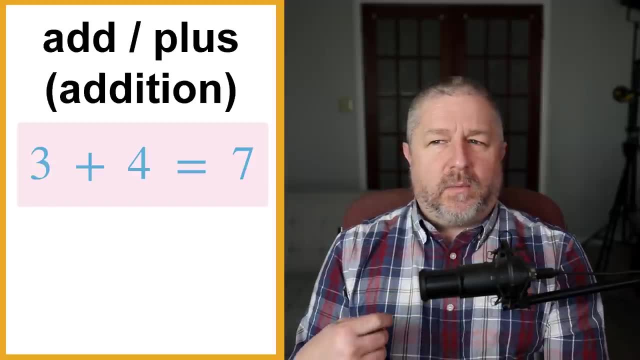 seven. So notice I'm throwing words in there and I'm using things differently. I'm saying, if I want to add two numbers, I would write an equation like this: If I wanted to add the number three and the number four, I would say three plus 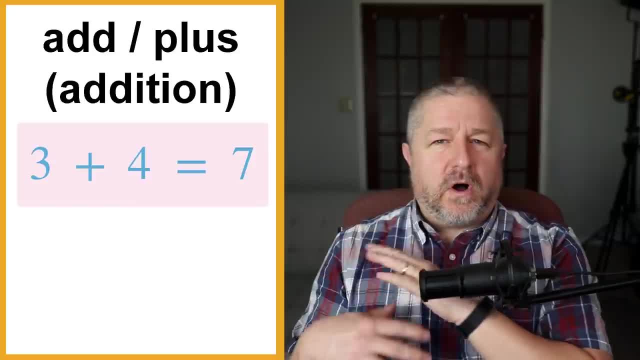 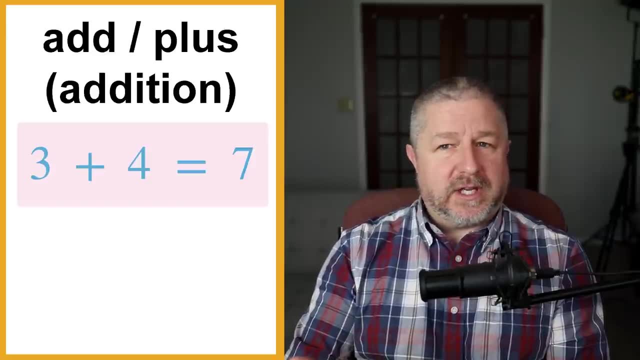 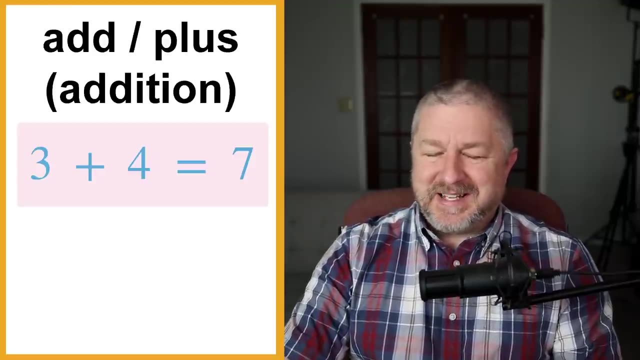 four equals seven. So we would refer to all of this as addition. when you're learning about addition in school, you're learning how to add numbers together, and you would do that by writing equations like this: Three plus four equals seven. Hopefully that made some sense. It's the add and the plus are. 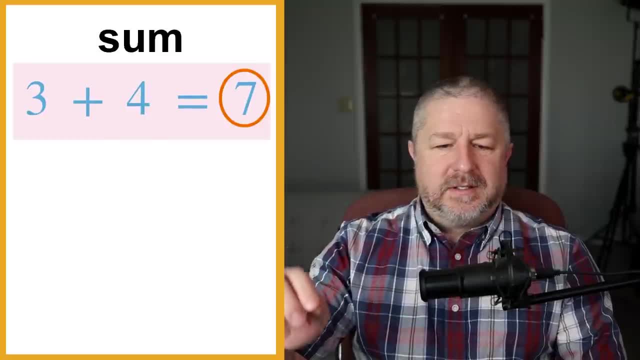 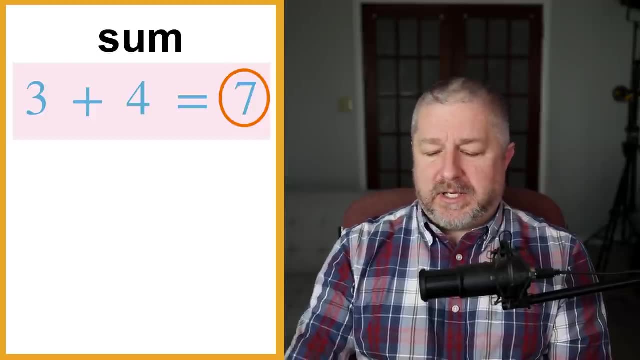 used slightly differently, if you've noticed- And then when you add two numbers together, you get the sum. So the answer: when you have addition, when you add two numbers together, the answer is called the sum, And then we have uh, subtraction. 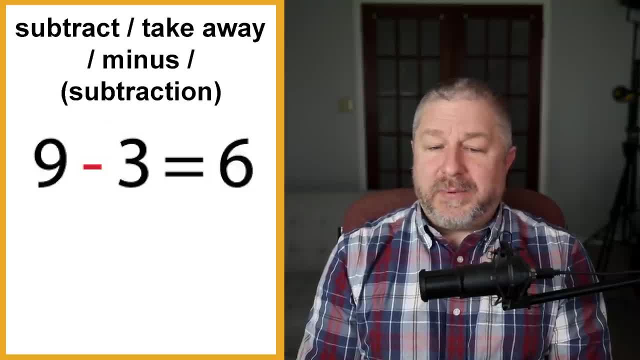 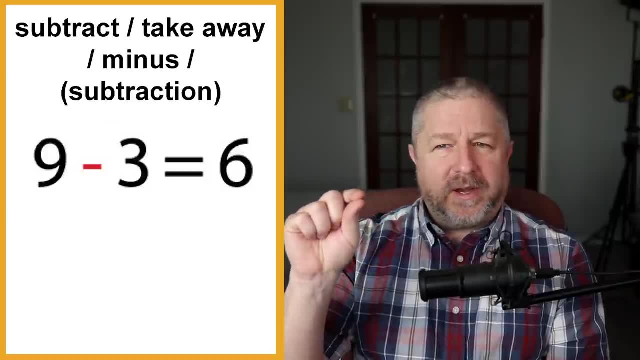 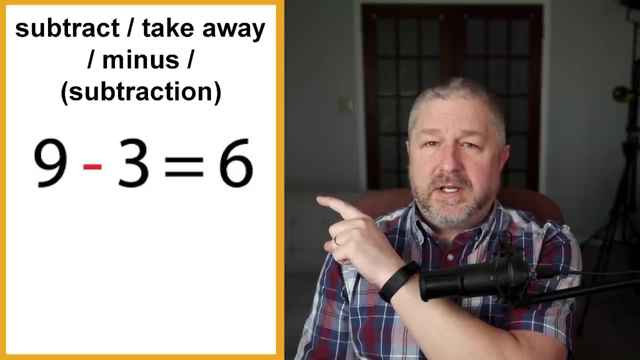 So when you subtract or when you take away or when you use minus, it's when you have one number and then you take a number away from it to get a smaller number. So in this equation I would say this: Nine minus three equals six. I could. 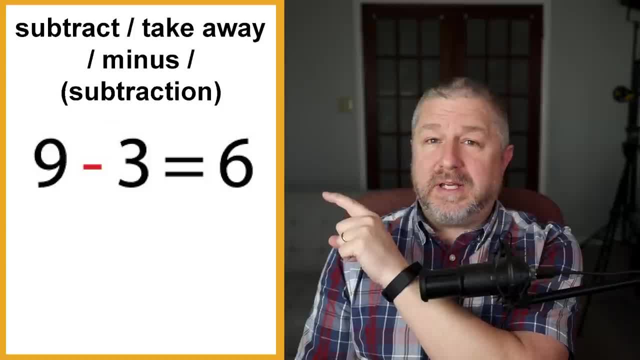 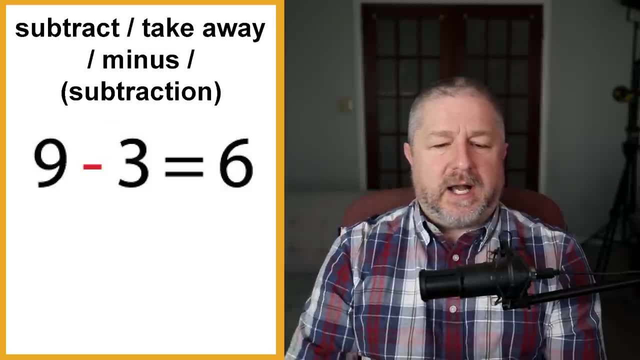 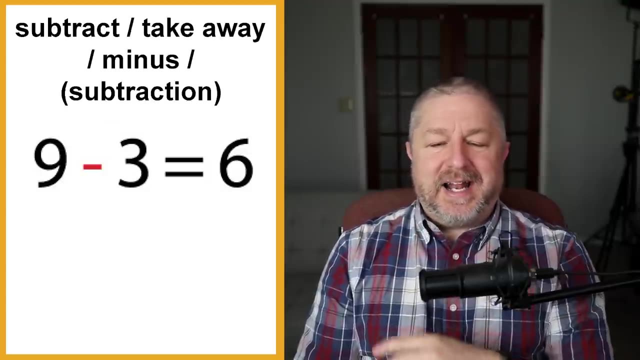 also say nine take away three is six, or nine take away three equals six. Notice, I use equals and is interchangeably when I talk about equations. Um, and I would use the minus sign. We could also say nine minus three equals six. That works as well. Uh, and again, we would refer to this as 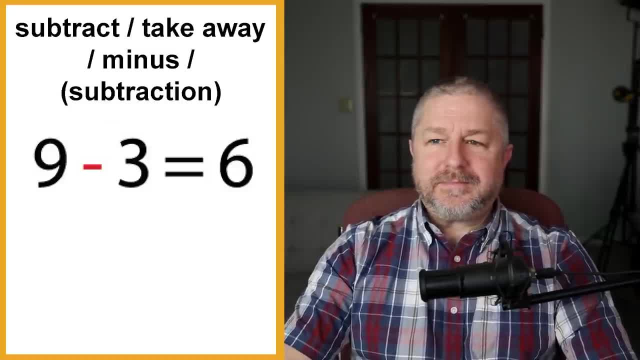 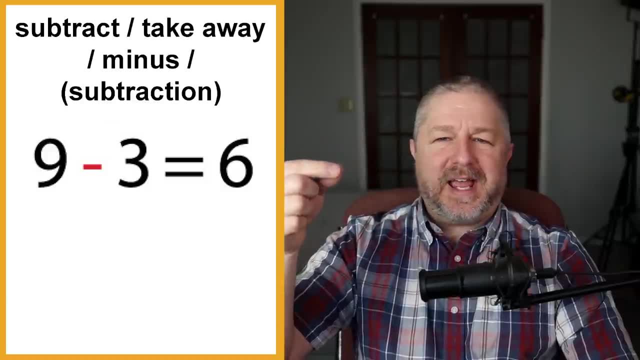 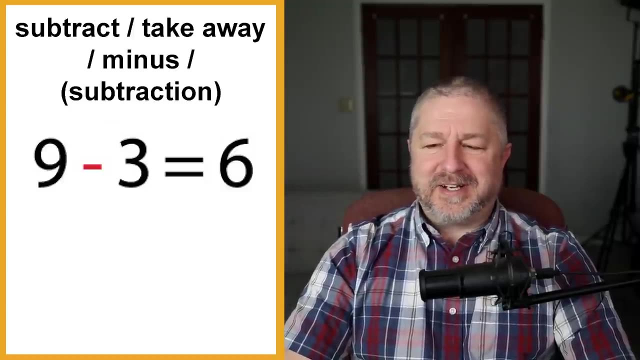 subtraction. When you're, um, getting paid at work, there's a lot of subtraction. You get a certain amount of money, but then, uh, they take money away for certain things like benefits and taxes. They subtract a lot of money from your paycheck And the difference, or sorry, and the 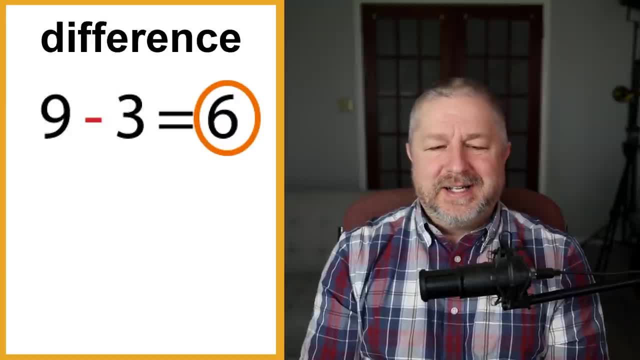 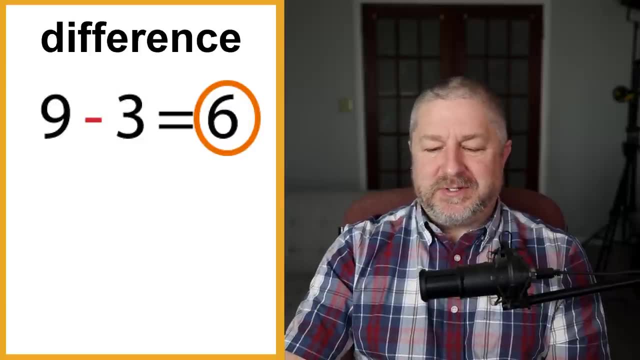 answer to an equation where you're using subtraction. Uh, the answer is called the difference. So nine minus three equals six. The answer: six is called the difference. I hope you're not getting too bored with this math lesson yet. Um, I, by the way, I. 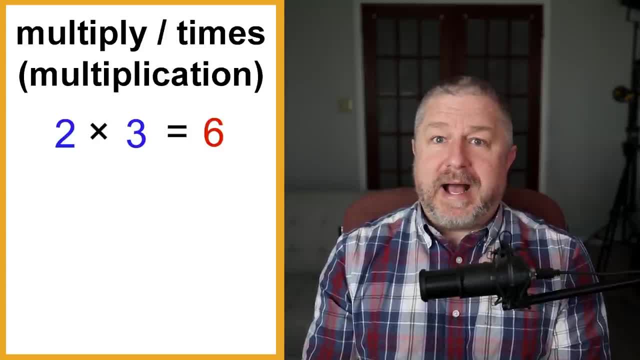 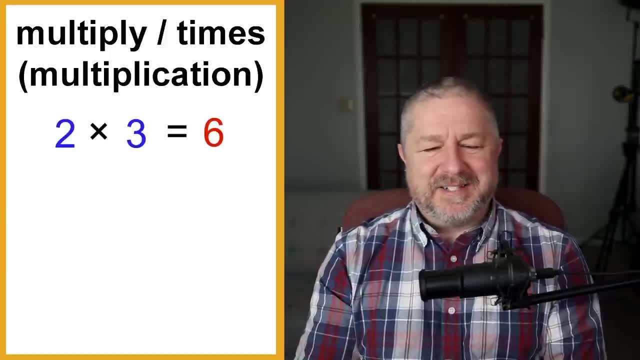 shouldn't say that, should I? I think there are a lot of people who love math. I myself do like math, So I'm I'm assuming for most of you, you're like me and enjoying this lesson. Uh, then we have, uh uh, another basic um function. uh, sorry, I shouldn't. 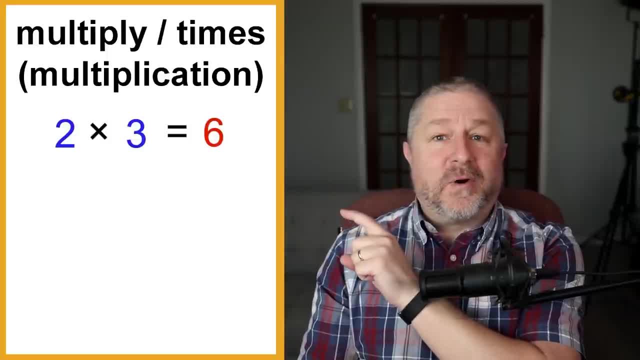 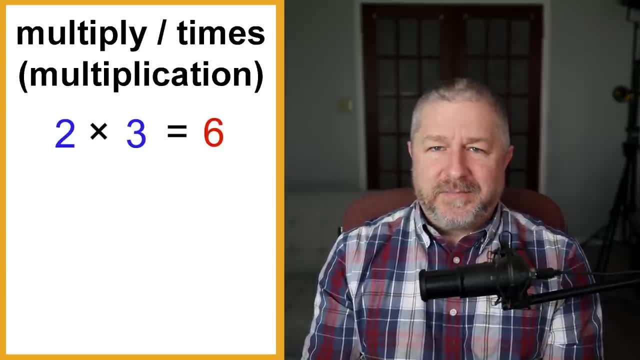 use the word function. That's a higher level math. Another uh form of basic arithmetic is to multiply or to use the time sign. So this is called multiplication. That's a hard word to say. I almost said it wrong. Multiplication is when. 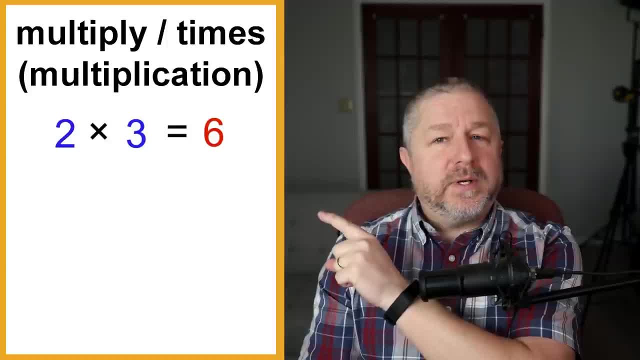 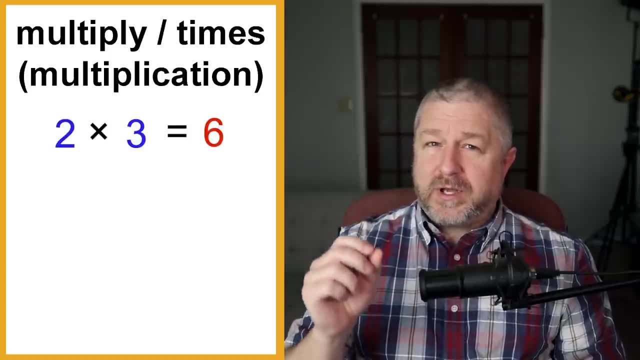 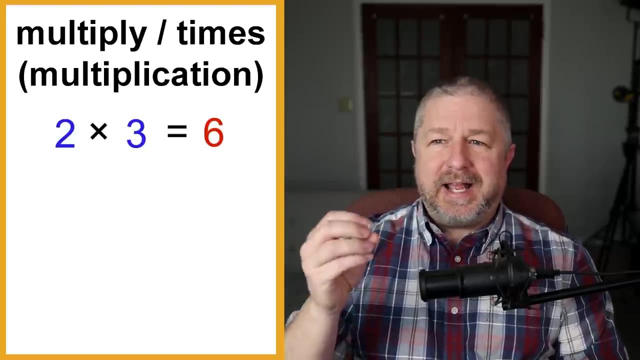 you take numbers like two and you say two times three equals six. So when you multiply two by three you get six. Two times three equals six. Notice how, just like add and um add, when I was talking about add and plus, multiply in times kind. 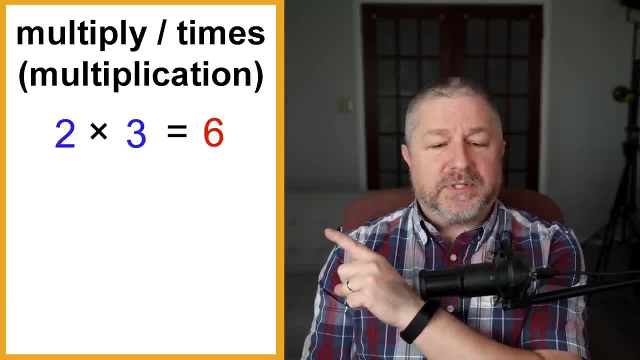 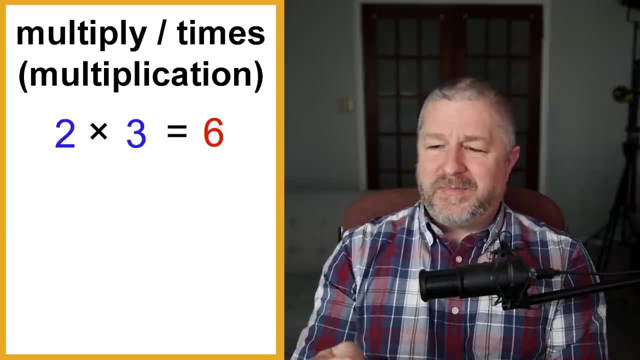 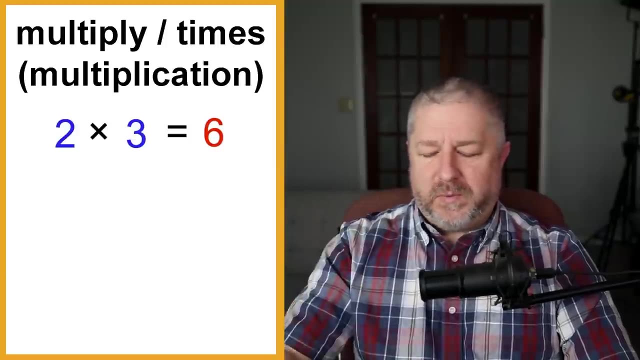 of work a little differently as well. Two times three equals six. This is a multiplication question, and in this question I will multiply two by three. I hope I'm not confusing you, but do note again that multiply and times are used a little differently when you talk about this equation. Let me say it: 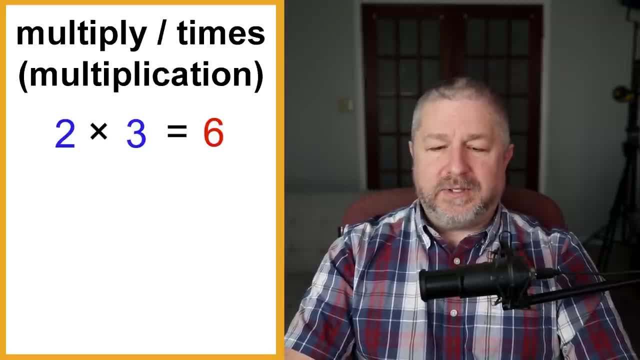 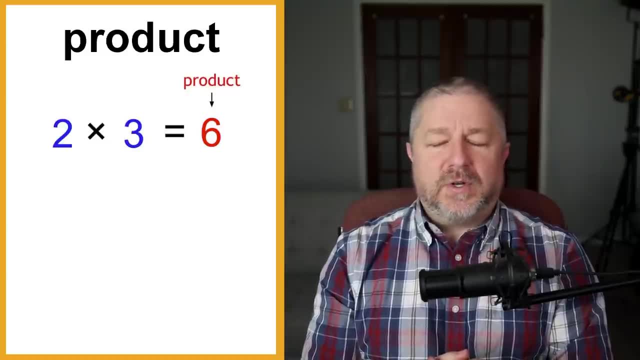 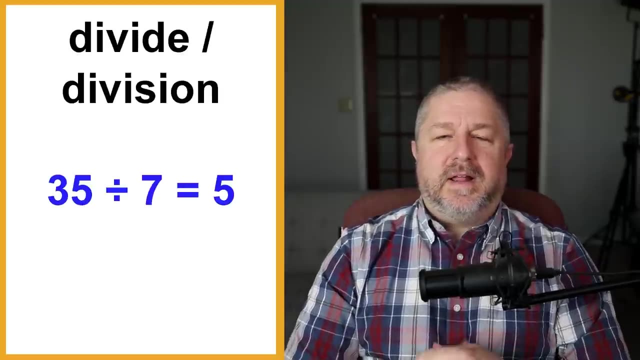 one more time: Two times three is six, or two times three equals six, And that is of course called a product. So the answer, when you multiply the answer to the question is called the product. Two times three equals six. Six is the product. And then we 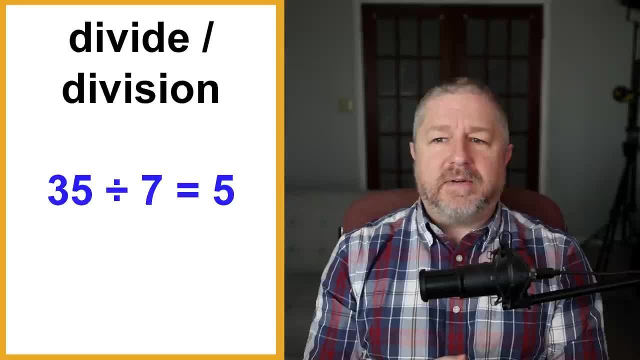 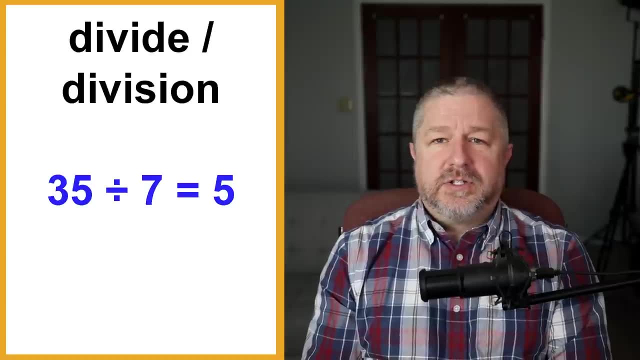 have uh division or when you divide. So when you have a number like thirty-five and you divide thirty-five by seven, you get the answer of five. So I would say this: This equation is an example of division. In this question I'm saying thirty-. 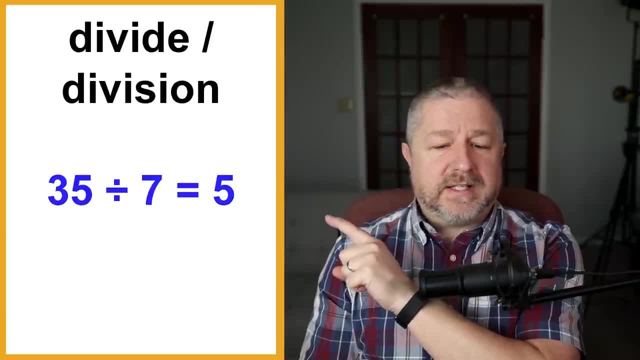 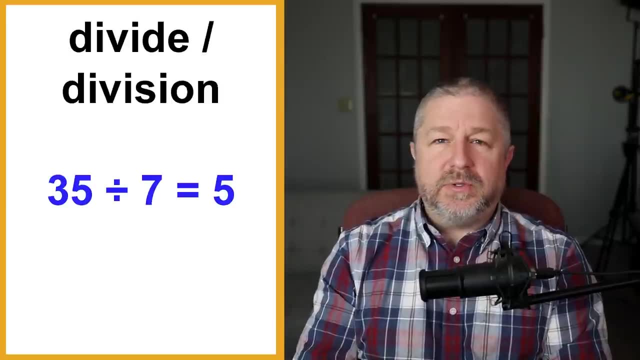 five divide seven equals five, or thirty-five divide seven is five. So again, we refer to it as division, but when we talk about the action that's taking place we use the verb divide. So thirty-five divide seven equals five. and the answer when? 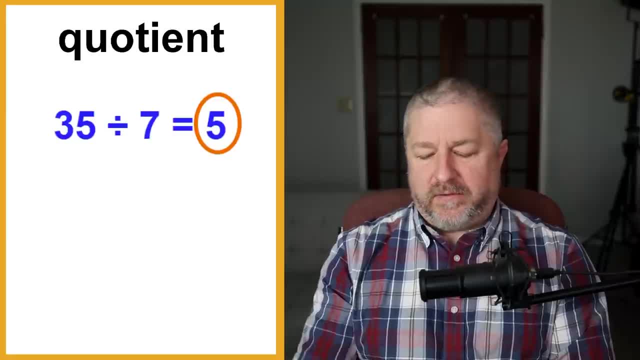 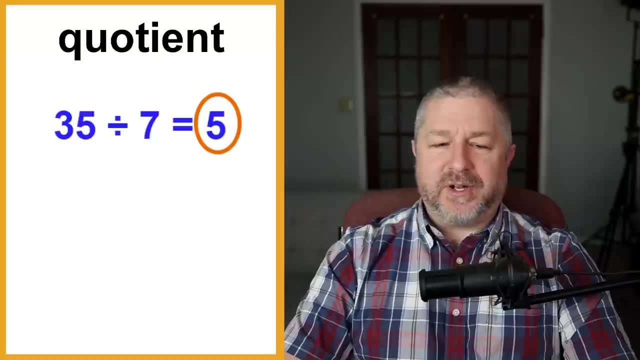 you're doing. division is called a quotient. So thirty-five divide seven equals five. Five is the quotient. So that was your basic arithmetic. Uh, should I go over it real quick one more time? No, Let's just move on. Nice and soft, Alright. 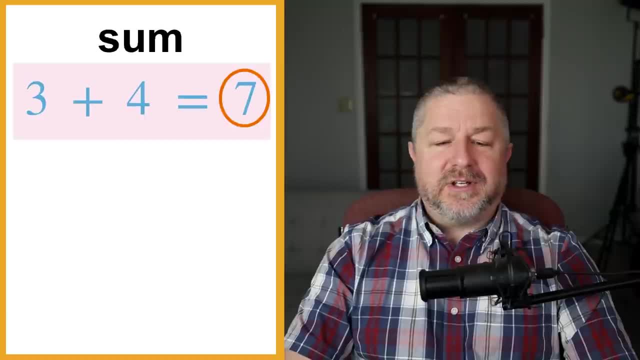 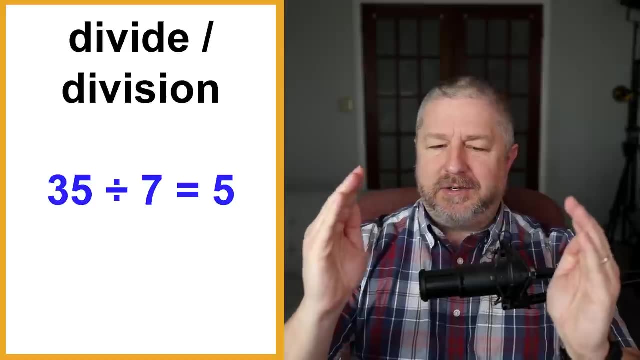 I'm going to pass this next question to you guys. I'm gonna on. No, let me go back. So you have, uh, addition, subtraction, multiplication and division. I'm not sure why I didn't put division in brackets. There was supposed to be like a visual. 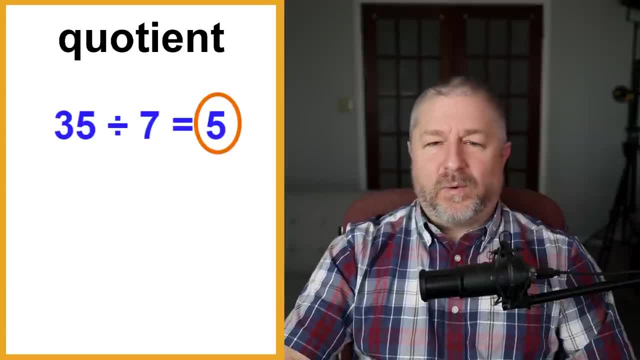 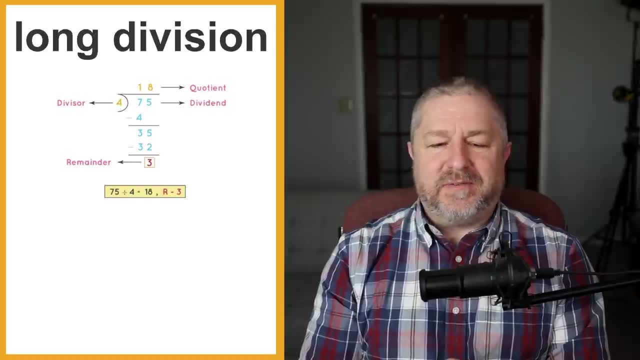 reminder for you. but anyways, those are the four parts of basic arithmetic. We also have long division. When you're talking about division, there are a couple of ways to do it. This is what we refer to as long division, where we put the 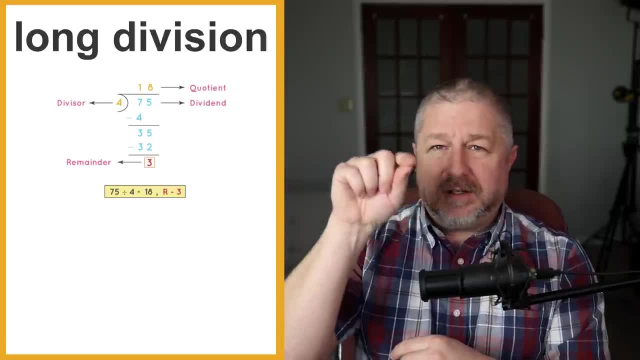 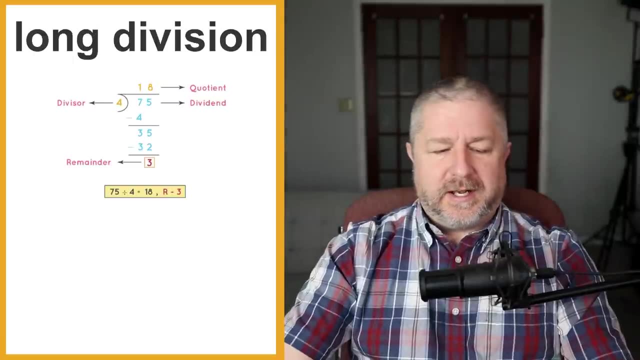 number, in the middle the dividend, and then we put this little bracket with a line kind of, and we have the divisor and then on the top you'll eventually get the answer, or quotient, I'm not sure if you like doing long division It. 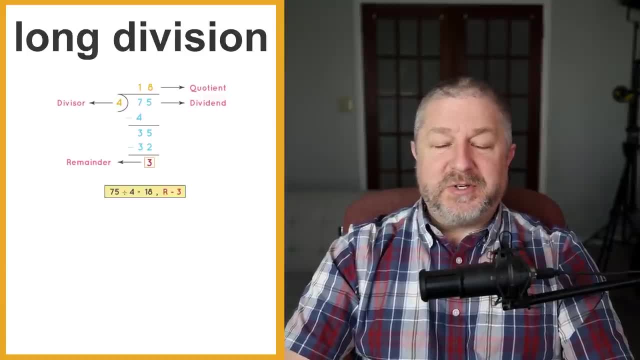 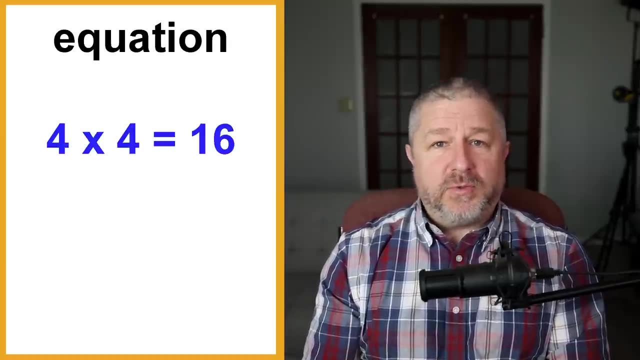 was one of my favorite things to do when I was in elementary school. Um, and so you've heard me use this word a few times. when you have numbers on a page with symbols like this, four times four equals sixteen, This is called an equation, okay. 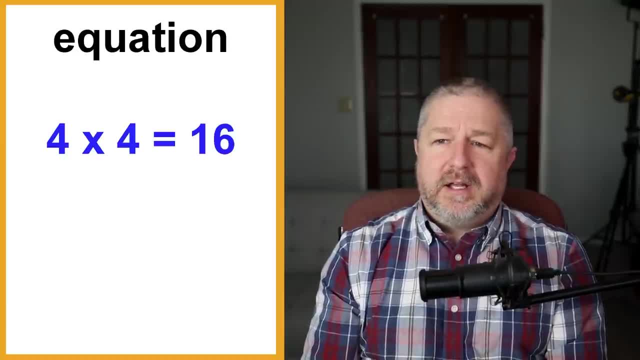 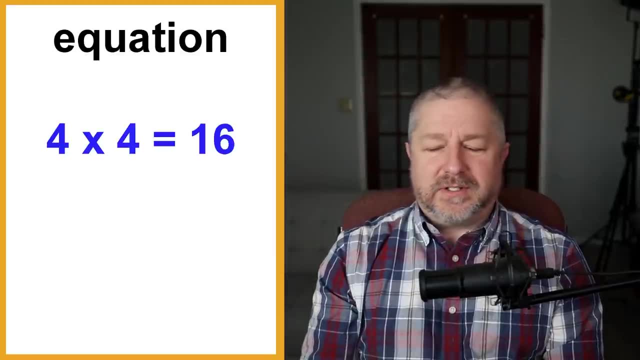 So when you go to school and when you learn math, you will have a lot of equations and there will be no answer and you will, in your mind, need to figure out, uh, what the answer is. So luckily, I can still remember that four times four. 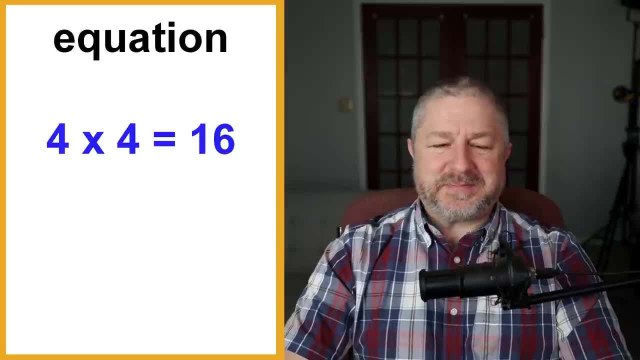 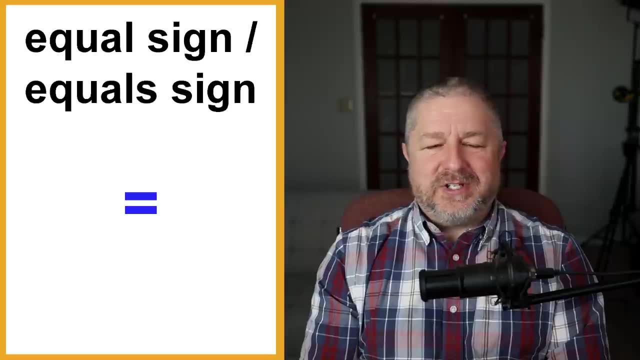 equals sixteen and that's an equation. Uh, and you'll notice that there is an equal sign or an equal sign in an equation. So the reason I have two spellings here is because, depending on where you are, you're going to have to do a. 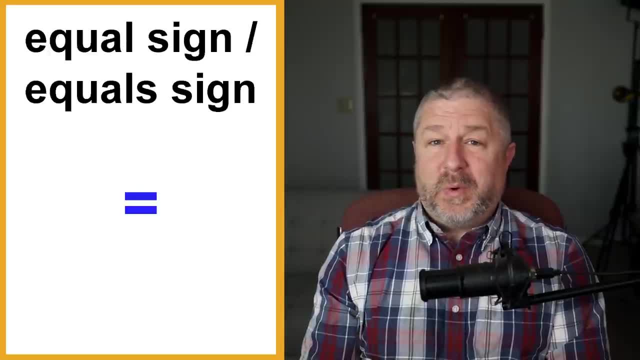 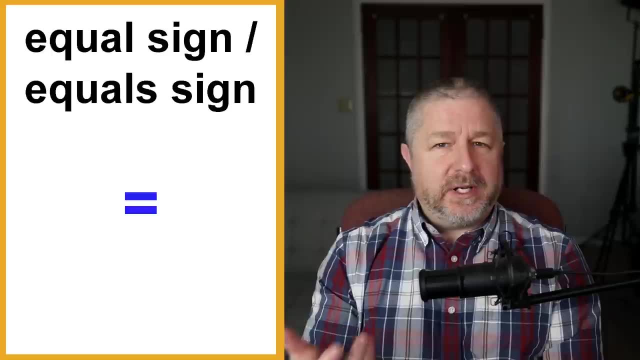 little bit of math. You might say one or the other. I use both, So I would call this an equal sign or an equal sign. but if you're in America you might say one, and if you're in Britain you might say the other. but Canada's kind of uh. 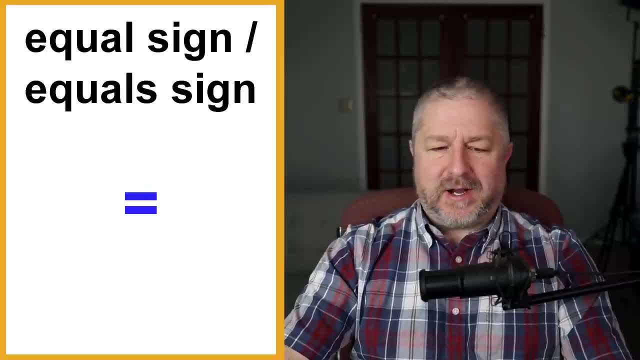 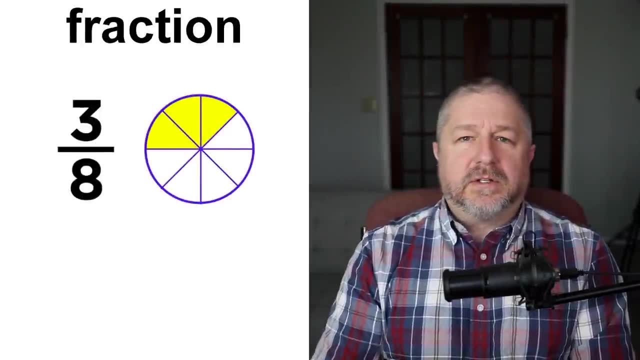 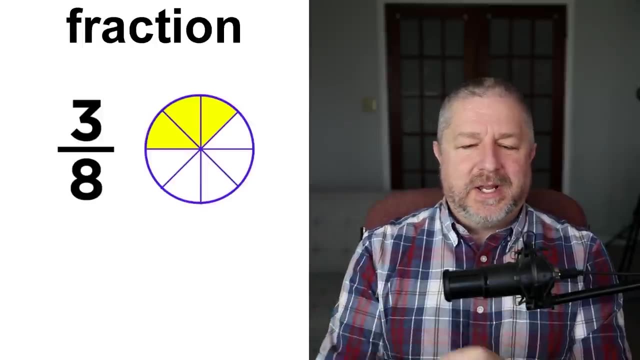 a mixture. Uh, Canadian English is kind of a mixture of the two, and so I use both of them equally. So we have what are called fractions, and a lot of times when kids learn fractions in school, we usually show them Graphs, or we we talk about pie for some reason, As you can see, 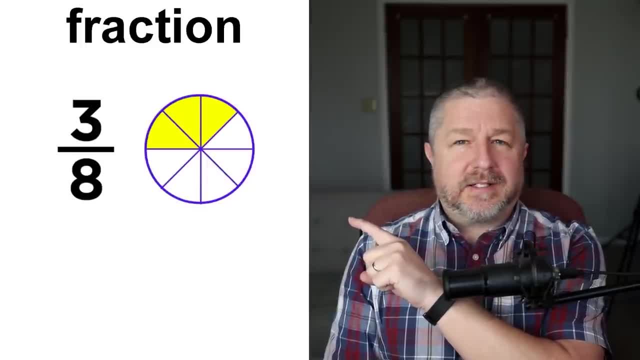 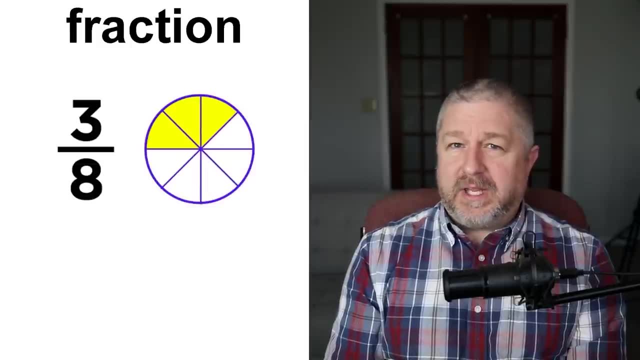 this pie or pizza has eight slices and three out of the eight slices are yellow. So we would say three-eighths of the pie is yellow or three-eighths of the pizza is yellow. I'm pretty sure this isn't a pizza or a pie, because I'm not sure. 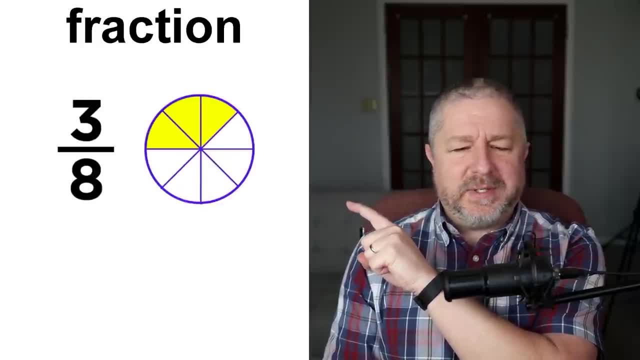 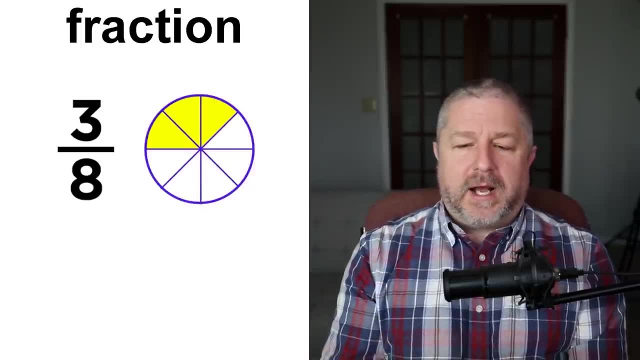 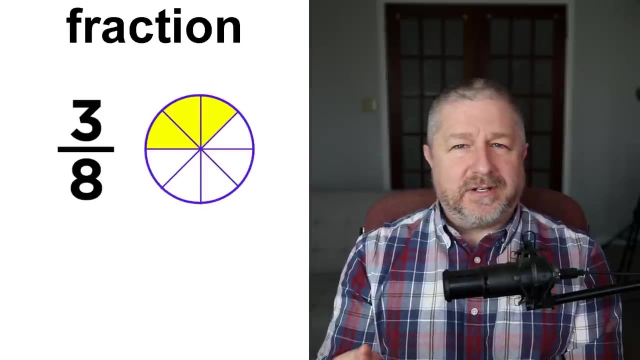 if any pizza or pie is purple with yellow pieces and white pieces. but a fraction is when you have one number on top of another number, A numerator on top of a denominator. Um fractions are still used, um because we use- uh, we don't use metric for everything, We still. 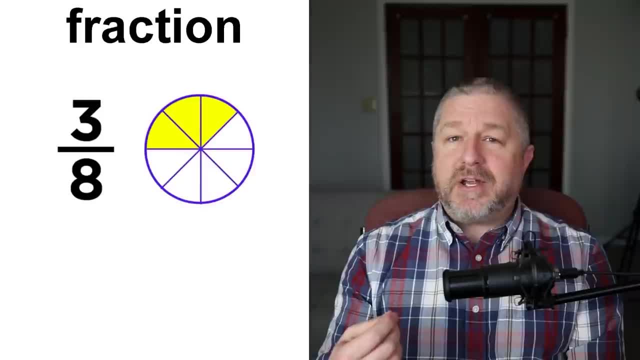 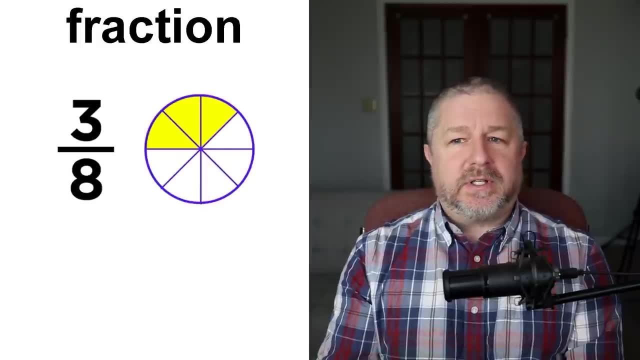 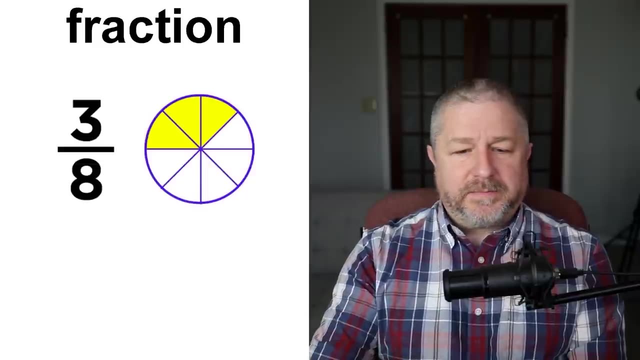 use what we call the imperial system. So we measure things in Canada in feet and inches because of our American- uh- neighbors. So we still use things like: you need to cut this board six foot and one quarter inches, or this board needs to be twelve and an eighth, So fractions are still. 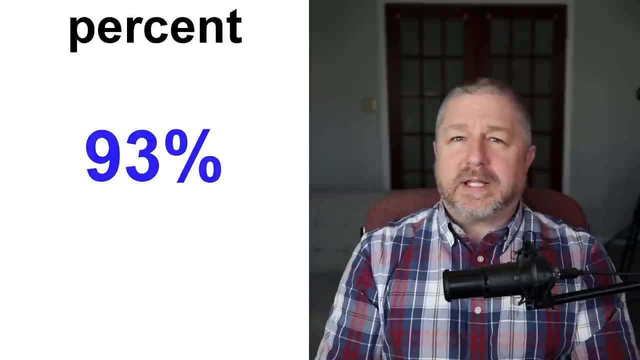 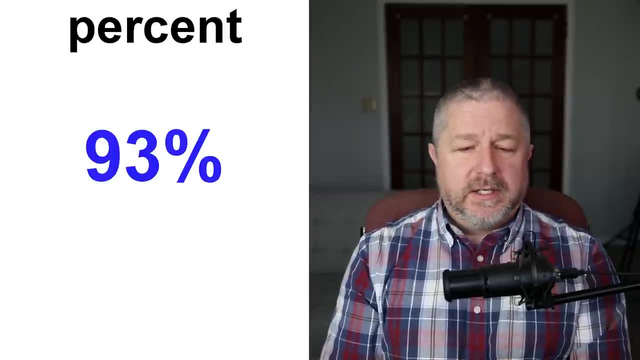 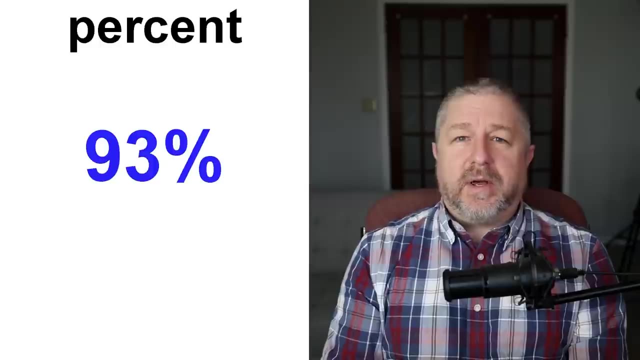 used, even though um. we've replaced them, I think, with decimals. in science and things like that. We also have the term percent. So when you have anything out of 100 um, which actually, if you look at percent, it has the French word, so 100 in it. So if you have a test and the test is out, 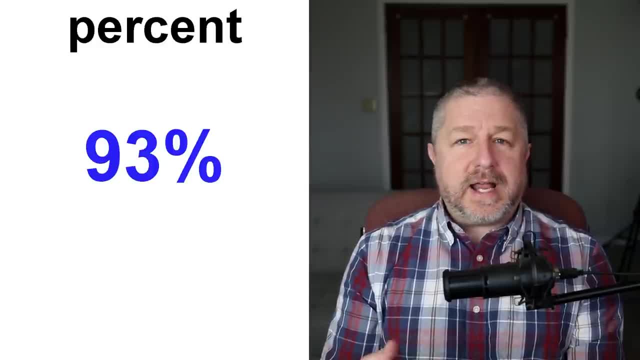 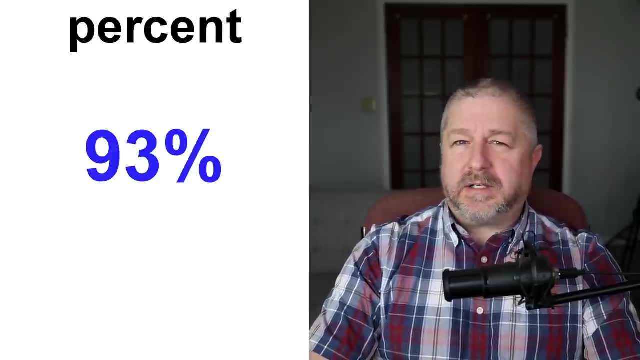 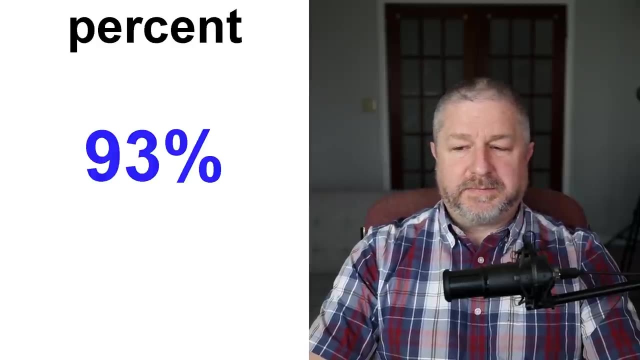 of 100 and you get 93 right, you would have 93% on that test. So percent simply refers to a number that is out of 100.. So a fraction is basically a fraction out of 100, but instead of writing it over a hundred, we just put the percent sign. 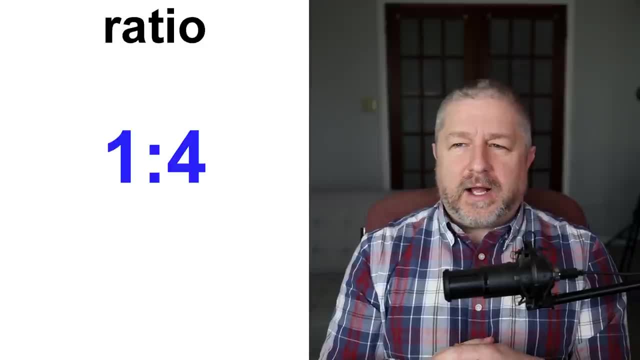 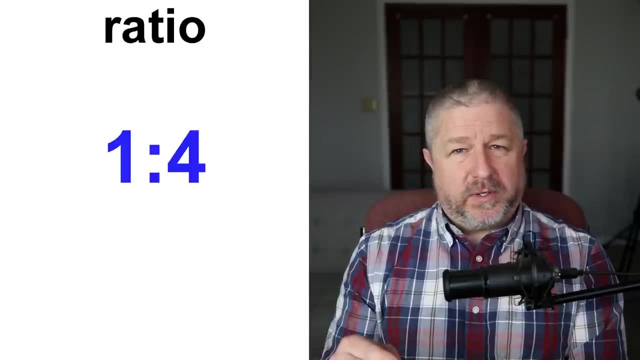 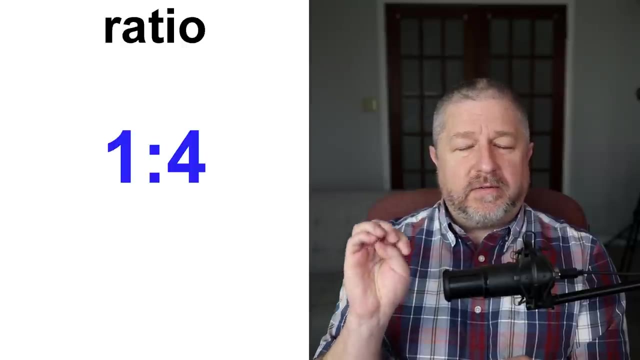 after it. Then we have what's called a ratio. So, uh, when I think about ratios, I think when I mix oil and gas, for my smallest lawnmower I need to mix oil and gas in a ratio of one to four. So I put one part oil for every four parts gas. 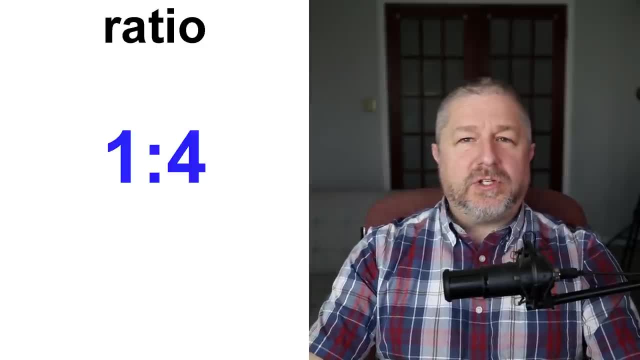 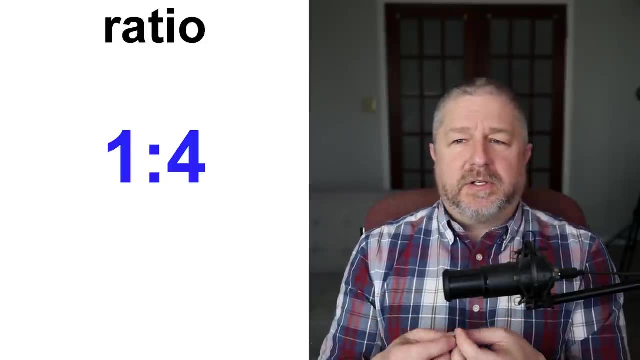 and I mix that together and that's how the engine runs. So When you have a ratio you're talking about, well, you can say things like this: How many men and women are at your workplace? And you could say, oh, we have a ratio of one to. 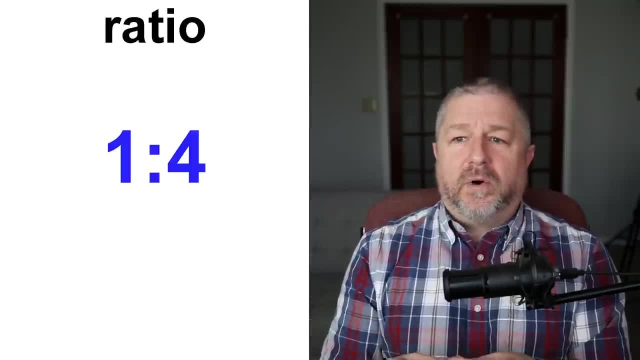 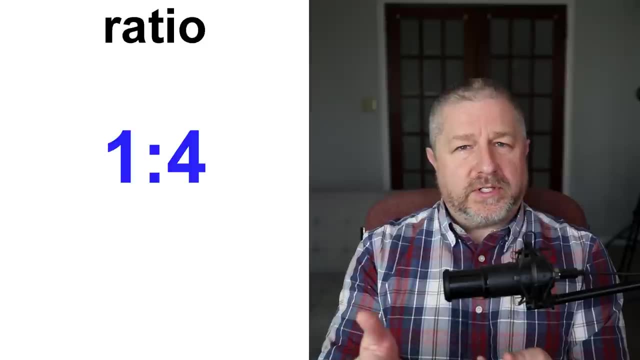 one For every man, there's a woman working at our workplace. Or you could say: oh, what's the ratio of students to teachers? You could say, well, it's about 30 to one. For every 30 students, there's one teacher in the school. So 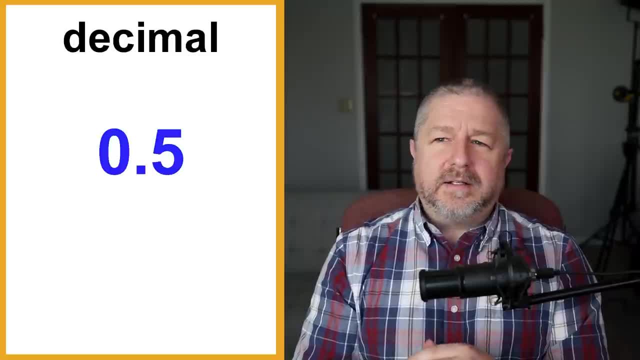 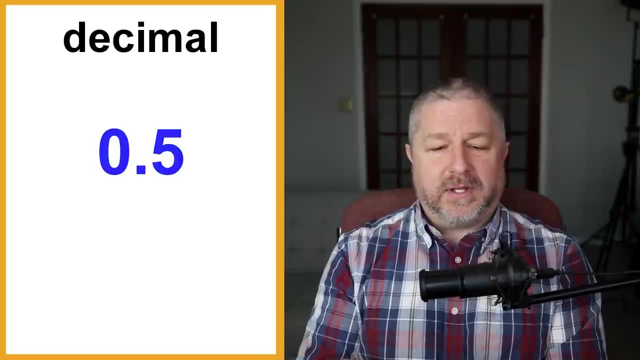 that's ratio, And then, similar to fractions, we have decimals. So if you have a fraction, one over two or a half, we would call it It is the same as the decimal point five or 0.5.. So 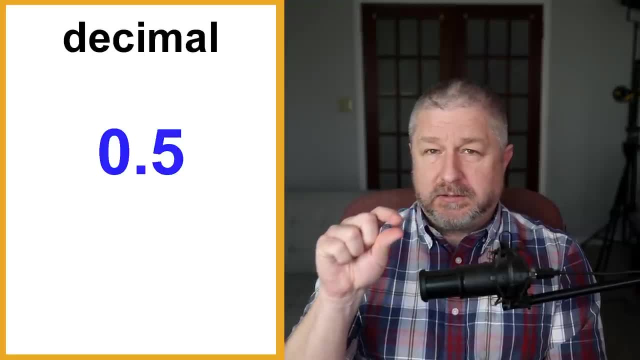 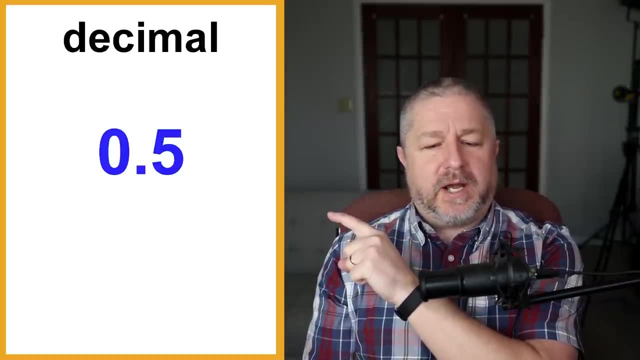 notice. in my part of the world we use the dot. In some parts of the world they use a comma as their decimal point. But for me, if I am going to write a decimal, I would write it this way. Um, if you want to, uh. 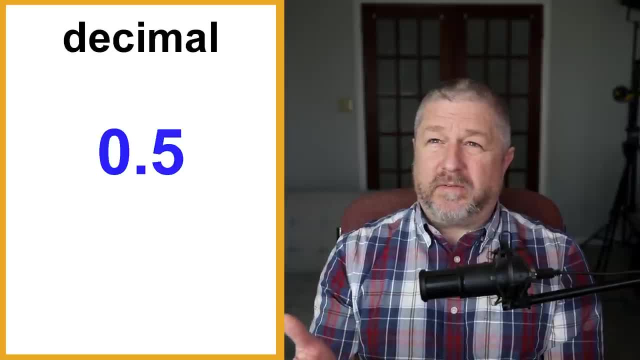 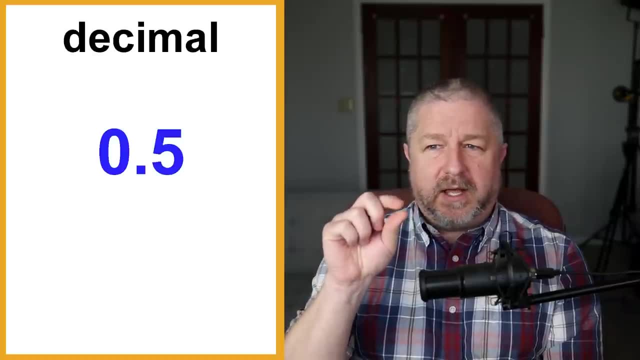 think of something like pi, which is 3.14159265.. Can't, I can't go any further. I used to be able to go further. Uh, there's a decimal point in um pi, So 3.14159265.. Yeah. 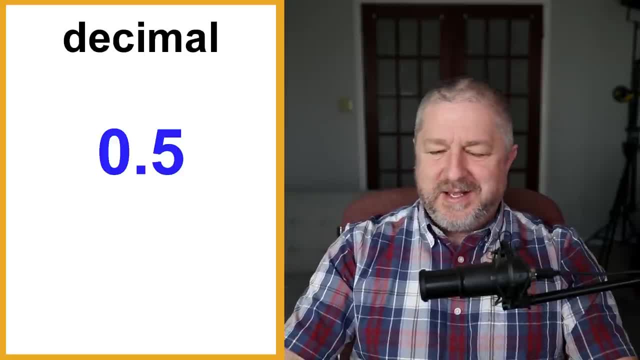 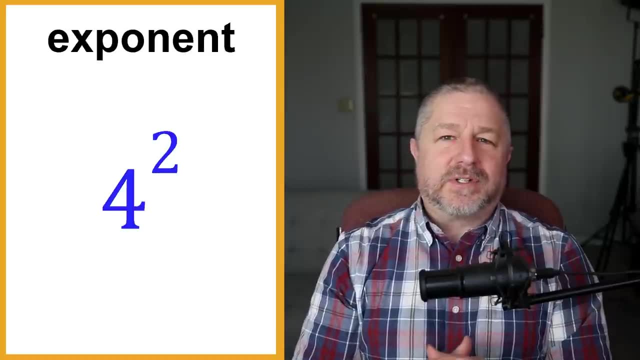 there's something, something eight, nine. Anyways, you guys can figure that out, Not going to try and uh, figure out pi to more than five or six decimal places. Um, and then we have what's called an exponent or exponents. So if you see, 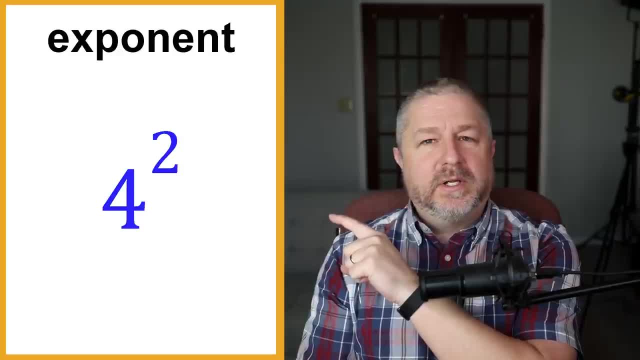 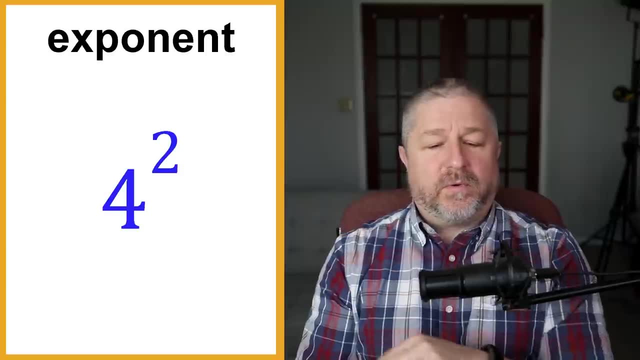 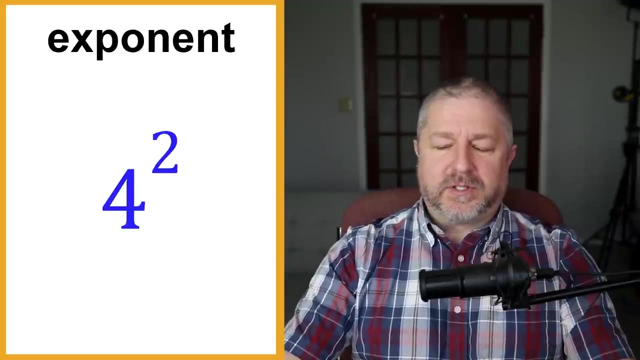 something like this In math: four to the power of two. The answer to this would be sixteen. It simply means that four needs to be multiplied by itself. So four to the uh, four to the power of two. when you have the exponent two, It means that you need to multiply it by 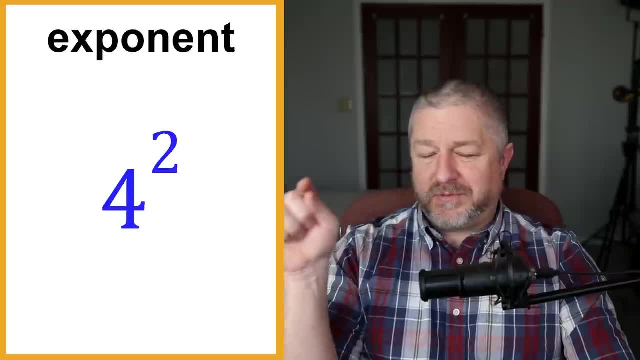 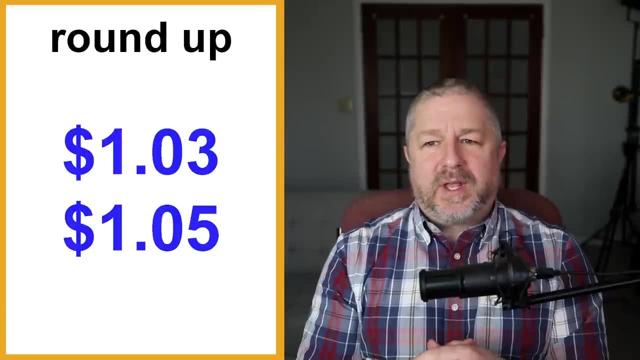 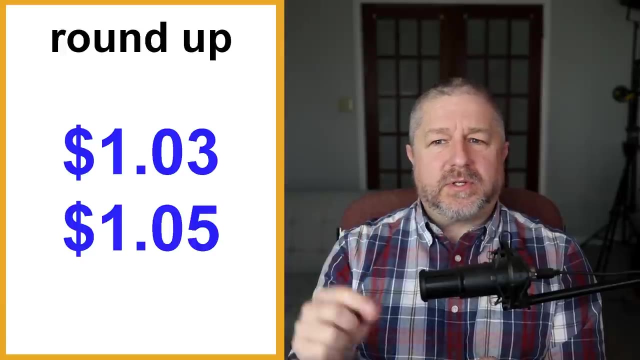 itself um two times. Well, once, really four times four. I think you know what I mean. We have something interesting in Canada where, uh, we don't have pennies anymore, We don't have a one cent coin in Canada, And so when you go to the store, 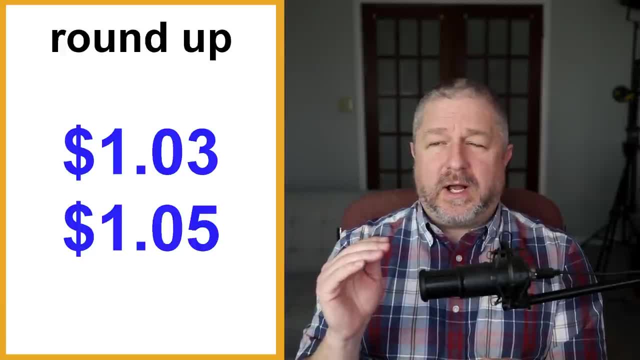 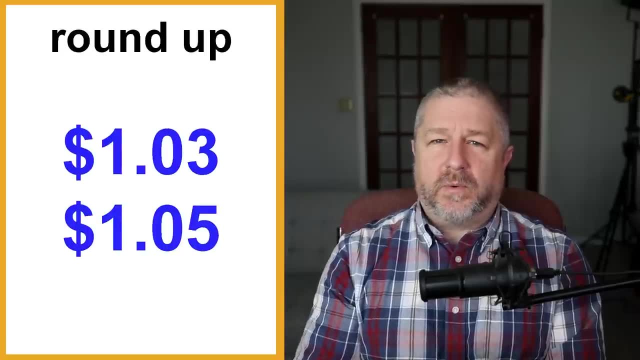 when you pay, it is always it's either- uh, they either need to round up or they need to round down to figure out what you owe. So if I go to the store and if I buy something and the total is a dollar three, If she says that will be a, dollar three. um, the machine automatically charges me a dollar five Because we need to round up, Because there's no, can't pay three cents. I can't give her a one dollar coin and then three pennies because we don't have pennies anymore. So 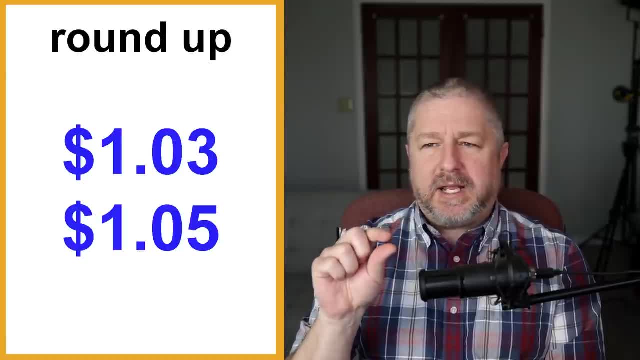 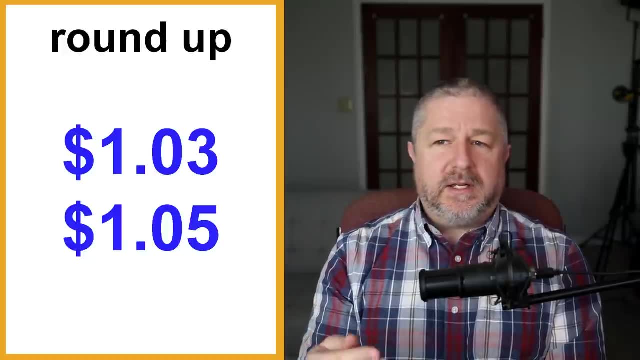 we round up. Round up is when you take a number and you bring it to the next highest number that makes the best sense for that situation. For us it would be to the next five cent point. So a dollar three becomes a dollar five when you. 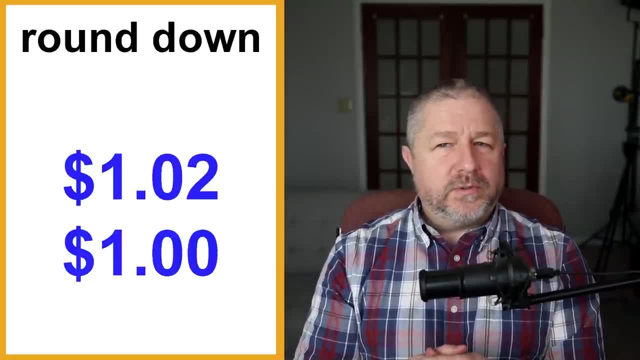 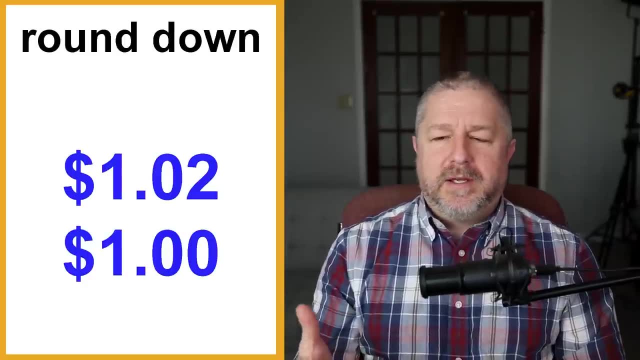 go to a store here and then a dollar two. this is where I'm happy, cuz I save a bit of money. A dollar two becomes a dollar at the store. So if I go to the store and I buy some candy and the total is a dollar two, I will be charged a dollar. 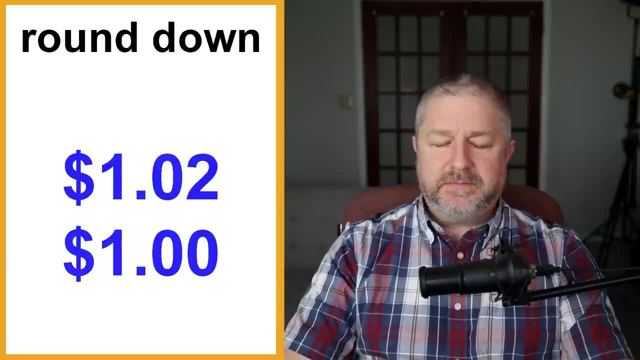 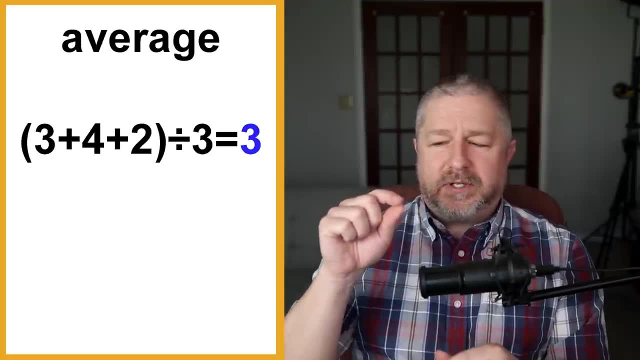 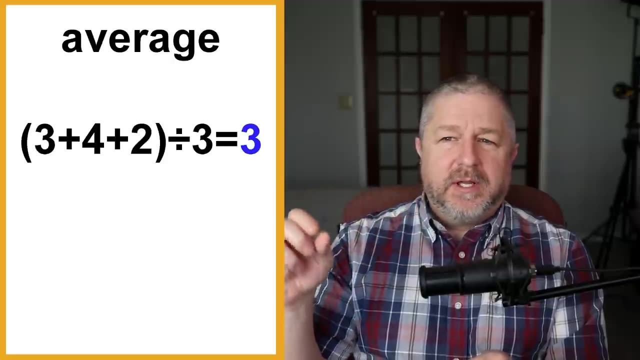 because they will round down to one dollar. Then we have something like average. So average is when you have a numbers, a few numbers in a row, and you want to know what the common average is between them. So let's say this, Let's say: 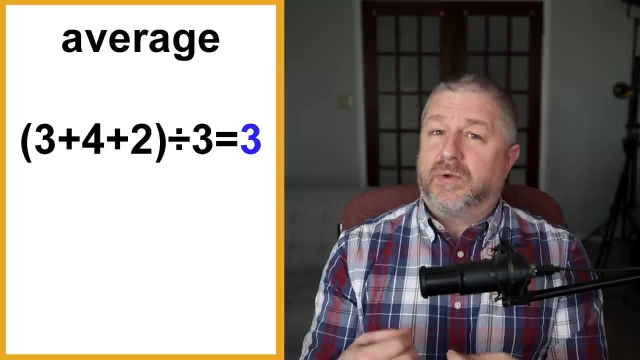 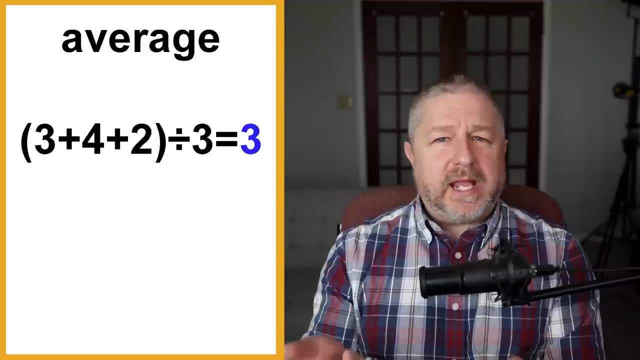 one day I sold three bouquets. The next day I sold four bouquets and the next day I sold two bouquets. If you wanted to know what's the average number of bouquets you sell per day, you would do this. You would add three plus four plus two and I put them in. 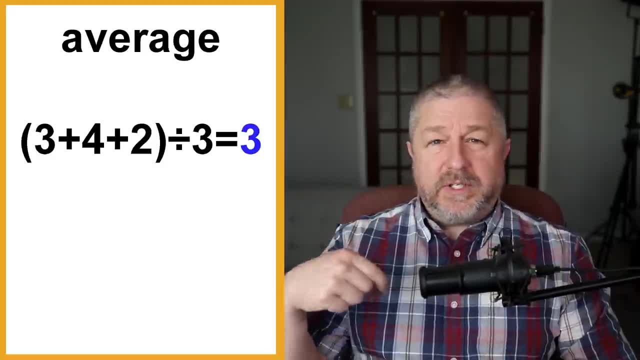 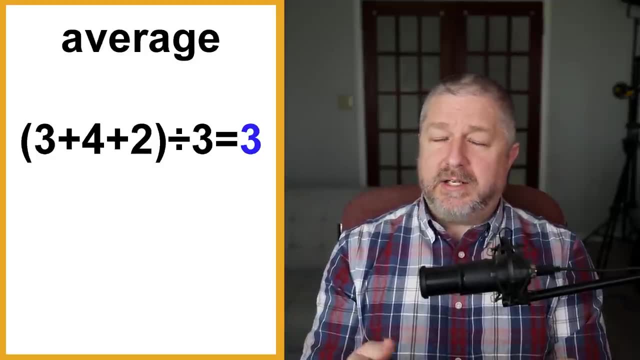 brackets, so that I do the addition first, and then I would divide that by the number of days. So divided by three, So it equals three. So three plus four plus two equals nine. divided by three equals three. So it means, on average I sell. 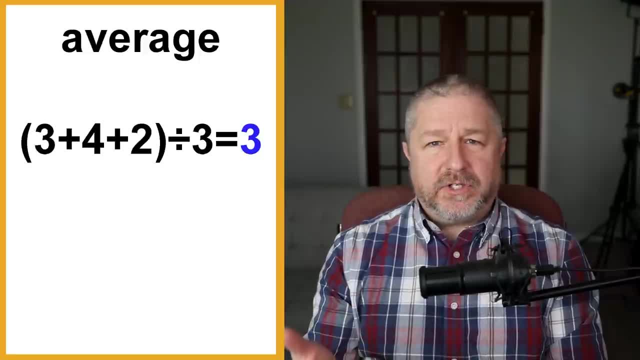 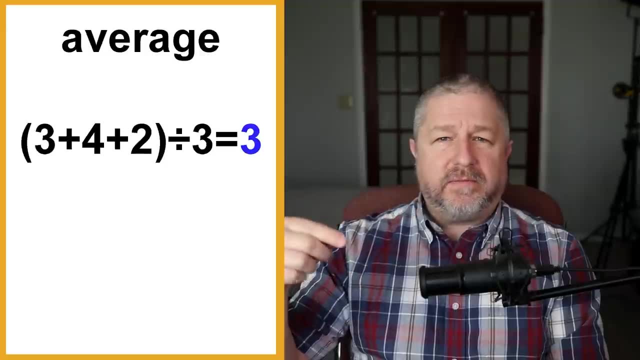 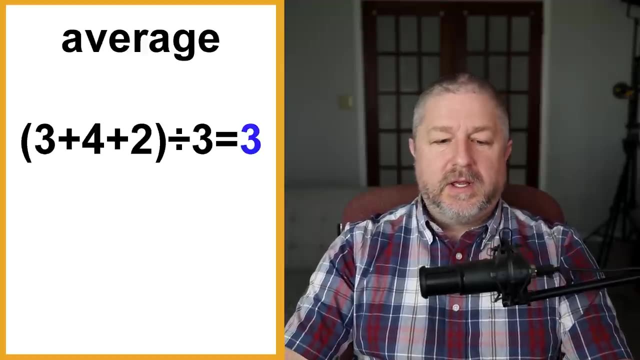 them per day. Students are always interested in knowing what their average is. They get grades for all the work they do in class and then they like to add them together and then figure out the average and that's their the grade they're getting for the whole class. So average, You'll notice I 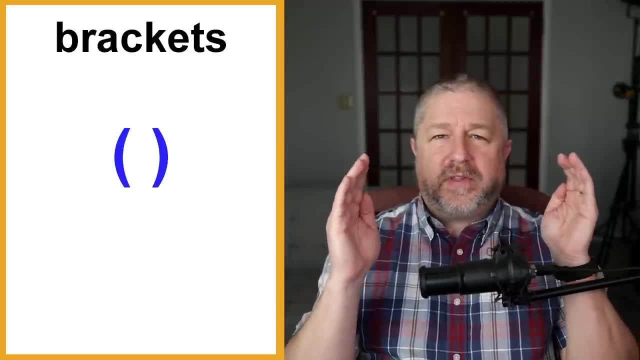 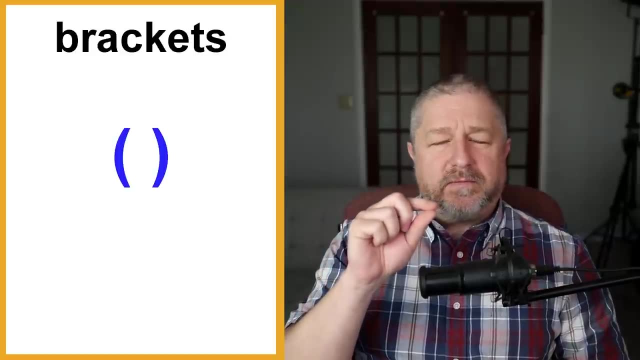 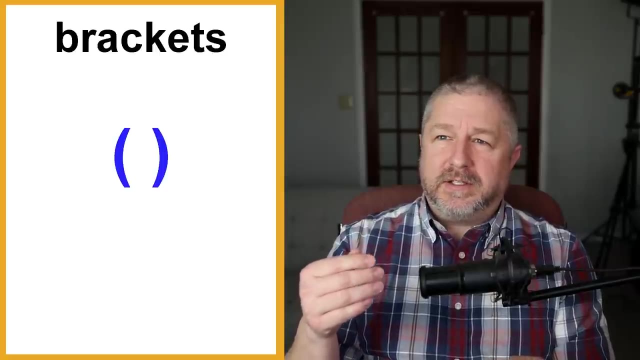 just used brackets. Brackets are these little curved things that you put in an equation in order to tell the person, that person- what things they should do first. Now there is a strategy. I think it's called bed miss, brackets, exponents. 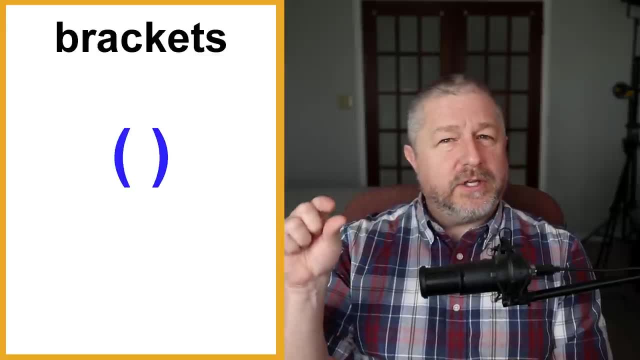 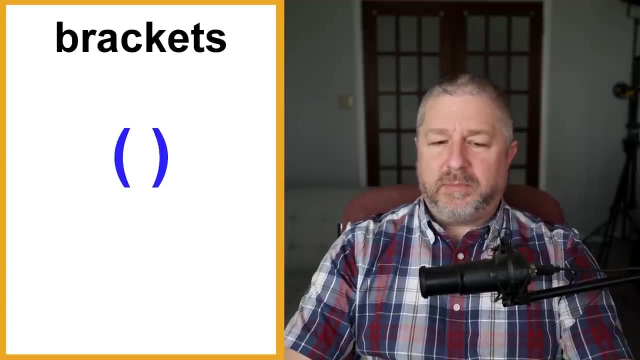 division, multiplication, addition, subtraction. There is an order that you're supposed to do, but when you put brackets in, you can indicate what order you want the equation to be solved in, because if there were no brackets in this equation, you could solve it wrong if you didn't know what order to do. 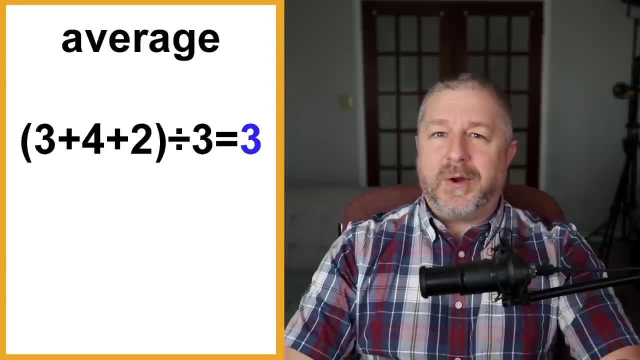 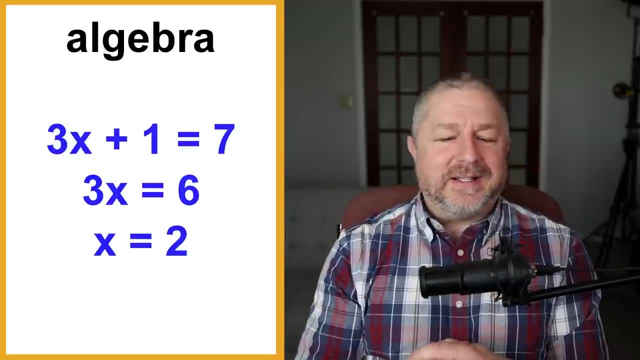 things in because the average wouldn't. it wouldn't come out correctly. Talking about math too much, I think I'm getting a foggy math brain right now. Anyways, let's talk a little bit about algebra. Uh, let me check where I am and then I'll pop into. 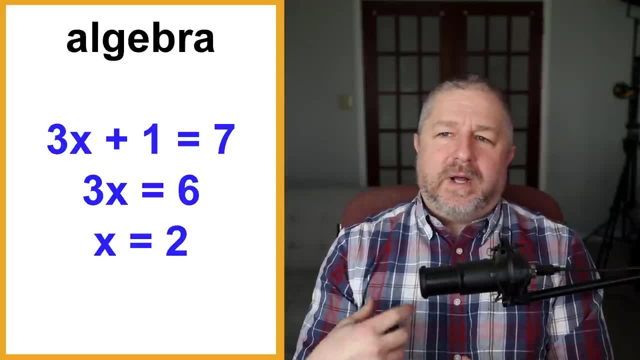 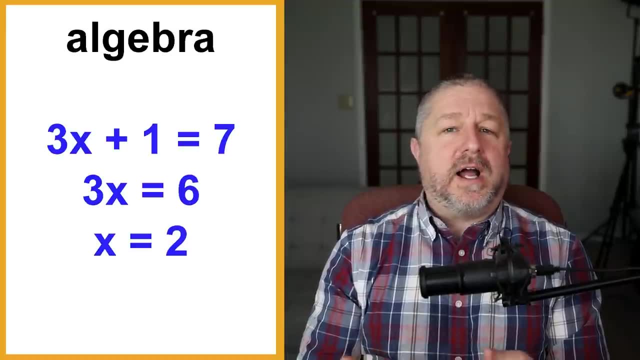 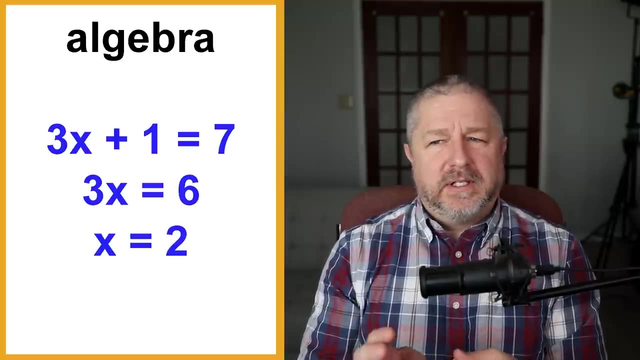 members only chat in a bit Algebra. So at a certain point in your math life you move beyond basic arithmetic and you start to learn higher level math In schools. in Canada students start learning algebra in about grade six or seven. They get a small 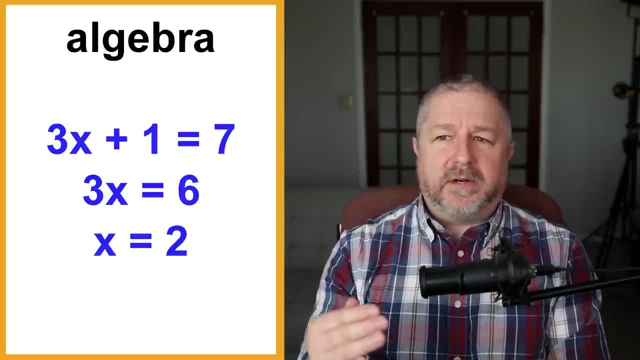 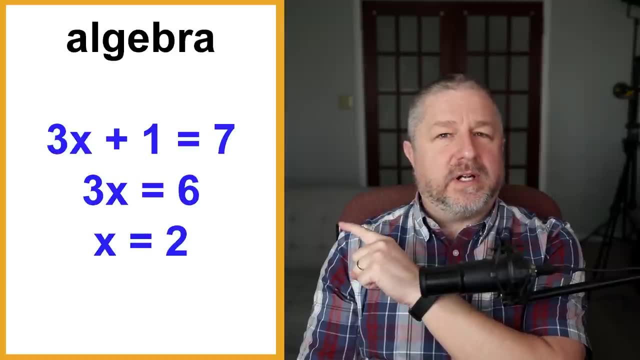 introduction to it, and they spend quite a bit of time in grade eight, nine and ten doing algebra and practicing algebra. So that's when you have things like this: You're given an equation: Three X plus one equals seven, and then you 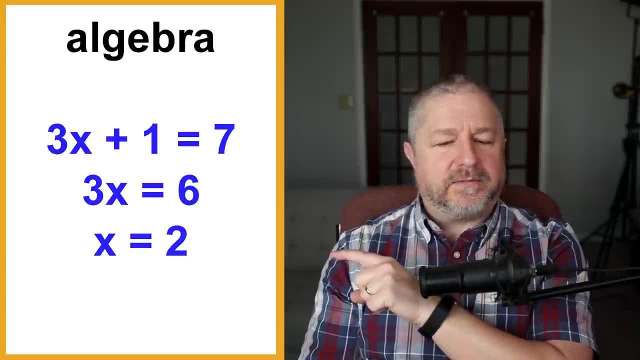 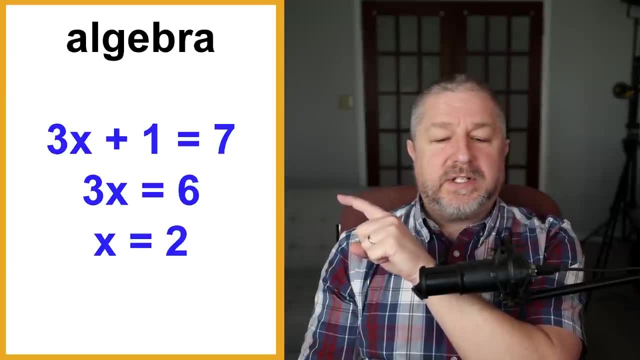 need to solve the equation Now. I've left out a step here. I left out the step where I move the three to the other side and divide six by three. but you can see here, three X plus one equals seven. That means three X equals six. 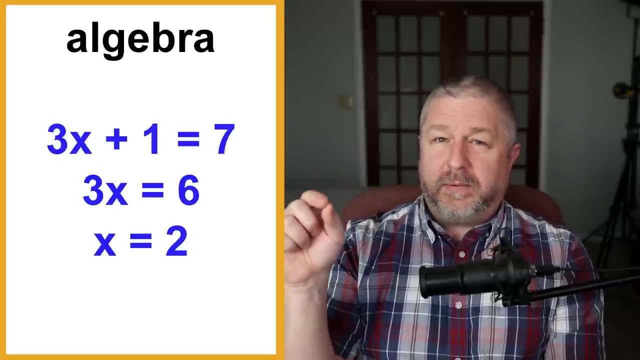 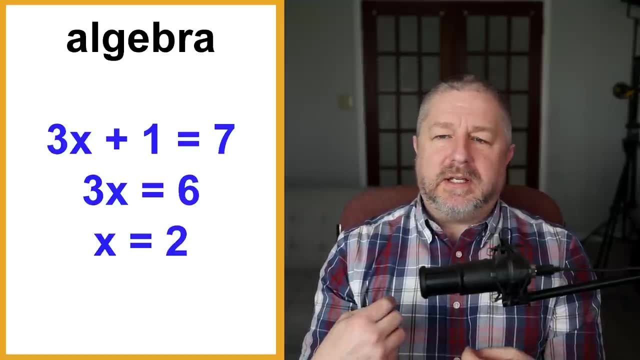 because if I move the one across, it becomes a negative. We get three, X equals six and X equals two. I might have left out two steps when I was solving this equation, but algebra is the, the study of math, where you have variables like the letter. 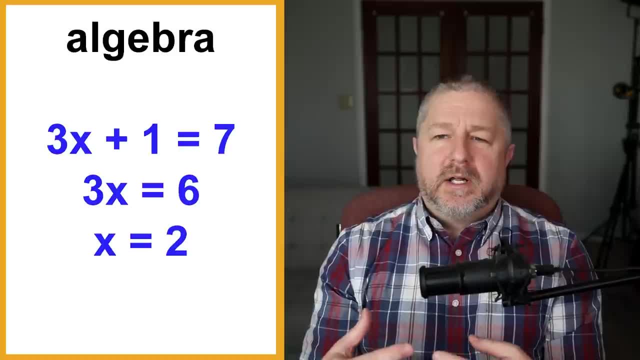 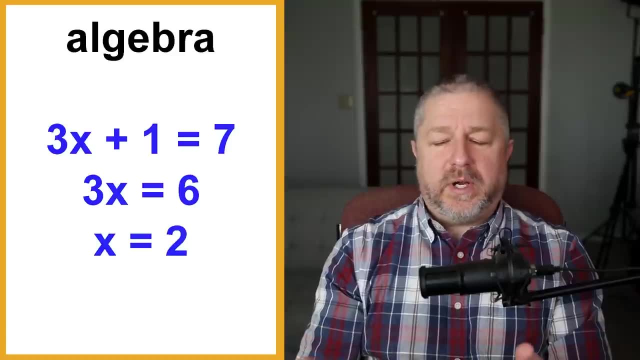 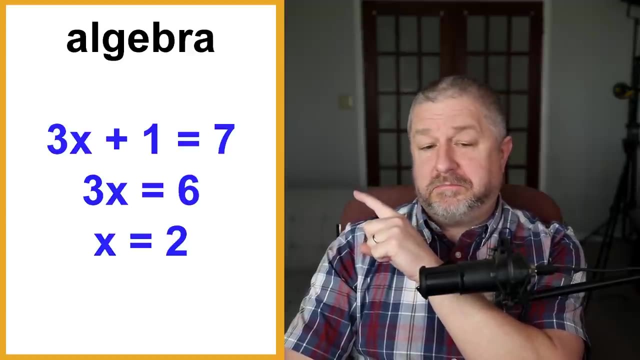 X is a variable. and then you have equations where you either are solving for the variable, or you're factoring or you're expanding. You're doing things with the equation in order to figure out different things. Algebra is a lot of fun. Hard word to say: maybe Algebra, Maybe not. 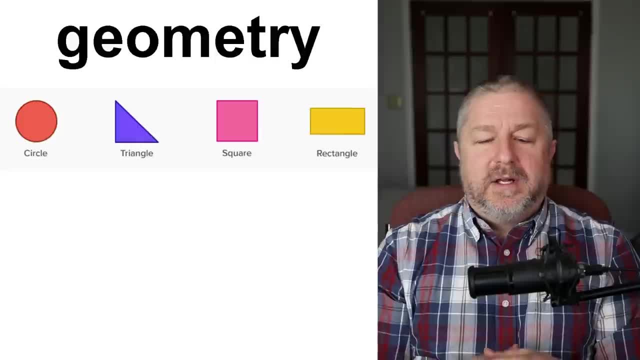 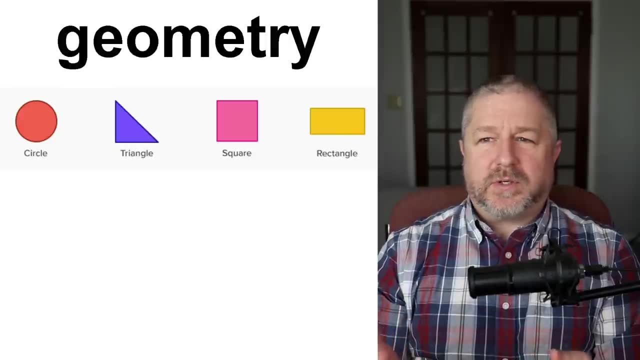 also have geometry. Let me make this a bit bigger. Geometry is an area of mathematics where you're studying shapes. So you're studying circles and triangles and squares and rectangles. You're learning about perimeter and area and you're learning about diameter and radius and those kinds of. 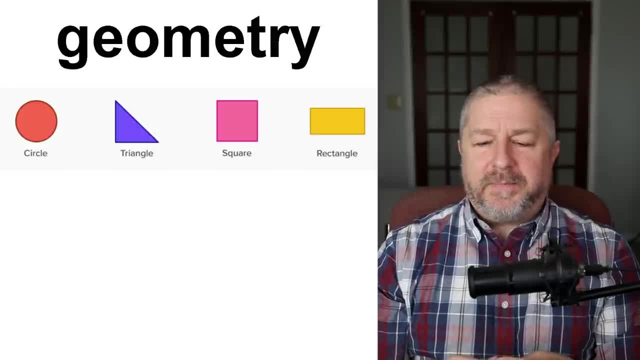 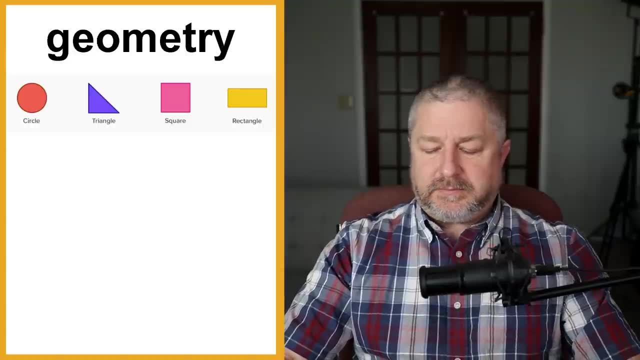 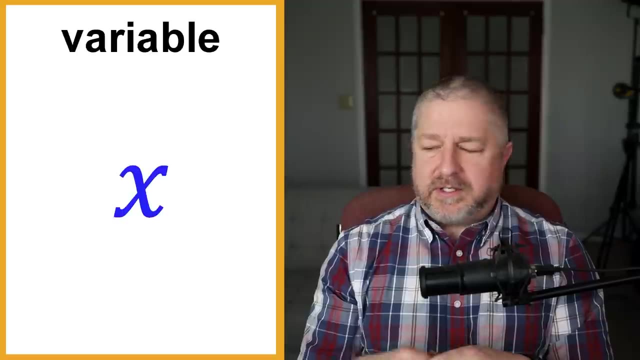 things. So geometry is the study of shapes. Um, this was also one of my favorite types of math. Geometry was a lot of of fun. And then I just mentioned the word variable. So in math, at a certain point, when you start studying algebra, you will start. 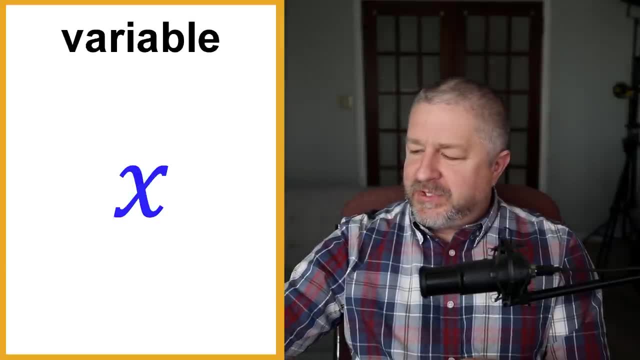 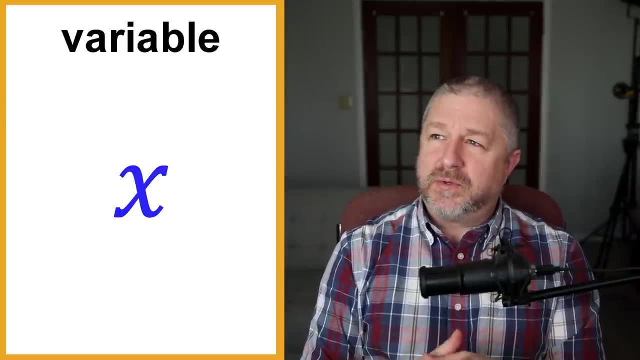 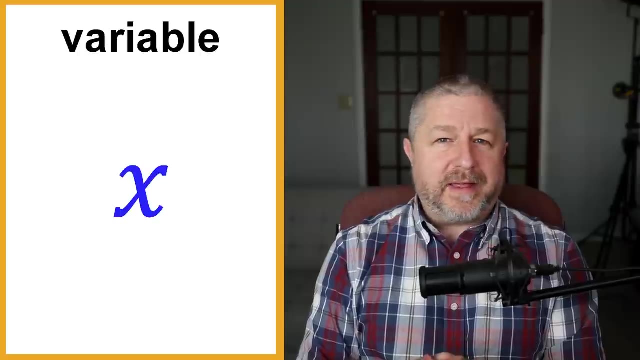 to see variables. You'll see equations like: minus seven C equals twenty-one. Then you'll have to solve that minus seven C equals twenty-one. That would mean C equals minus three, I think. Again, don't quote me on this, I am not a math expert. 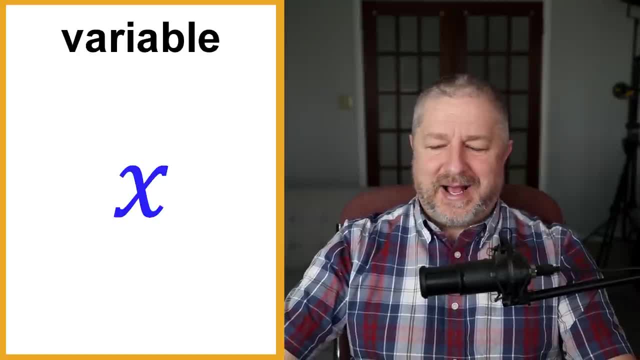 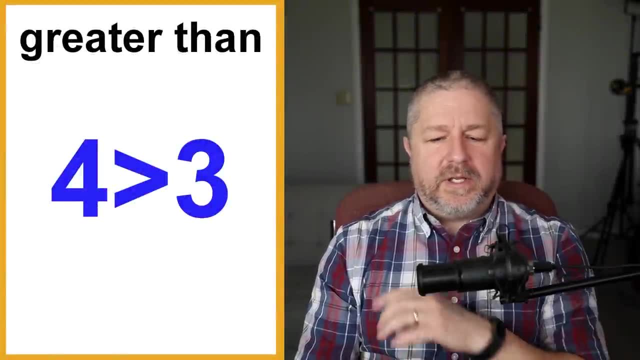 could I? I'm not a math teacher, But I do remember some math from my life. So we saw some of this in the chat already. We have the greater than sign. When you see something like this, you would say that this is true: Four is greater than three. The way 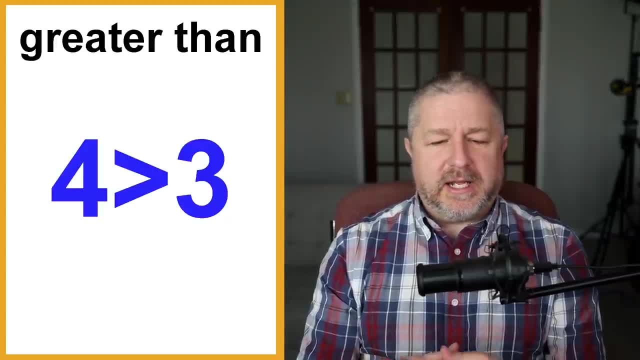 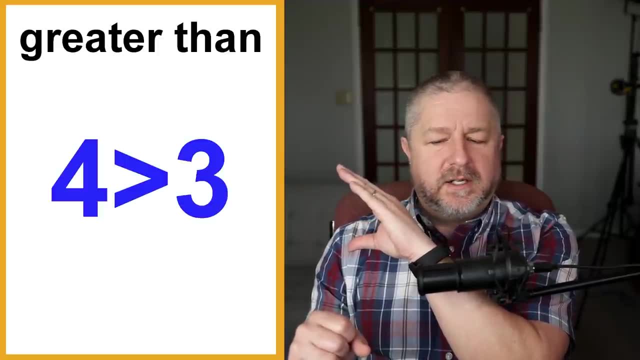 they taught me in elementary school. the way to remember this is that if you picture the greater than sign as a mouth, they always said to pretend it's an alligator. The alligator always wants to eat the bigger number. That's the. That's how you know which way to put the greater than sign. 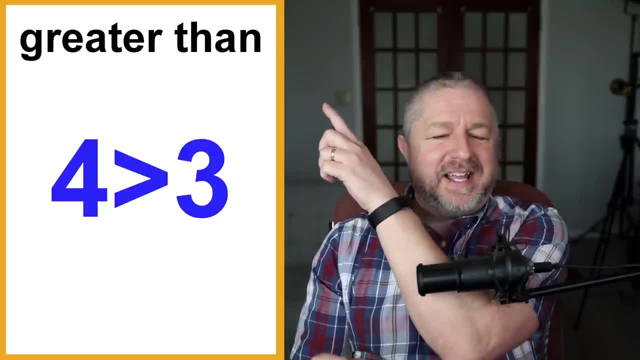 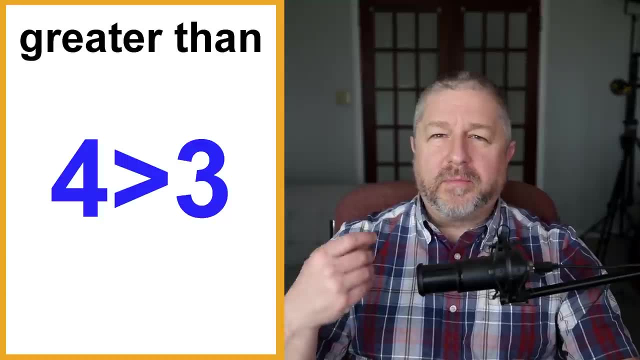 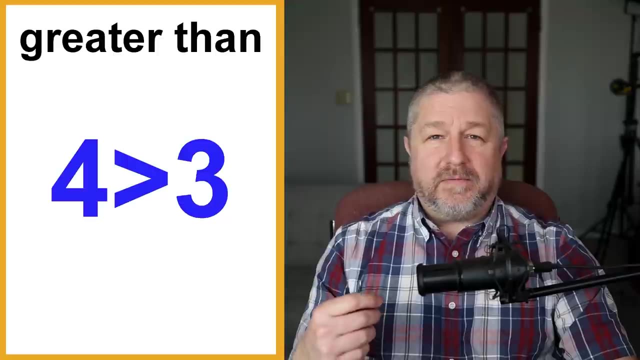 And notice up here it's than T-H-A-N, So that is a greater than sign. Four is greater than three. I'm over pronouncing than right now When we say than really quickly it does sound like then. So I would say four is greater than three If 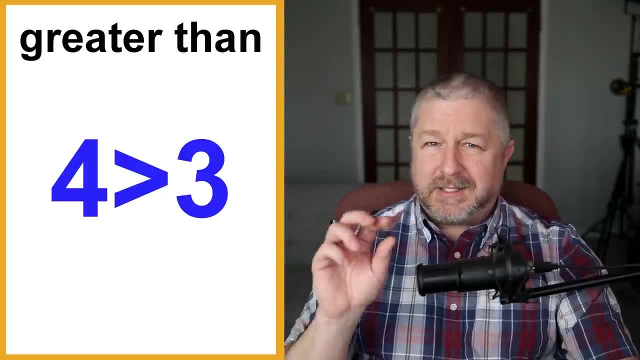 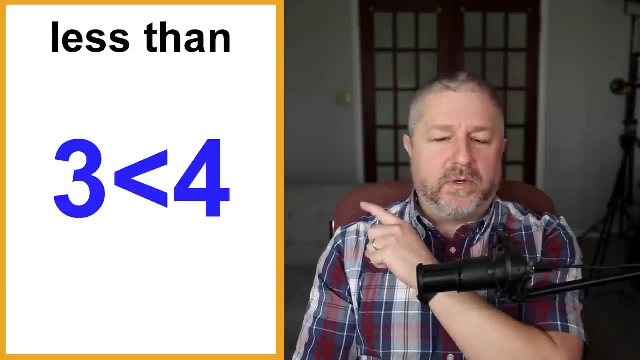 I say it fast. I would say four is greater than three, And it sounds a little bit like then, but it is than, And of course we have less than. So three is less than four. Notice, the alligator is trying to eat the bigger number again, So again. 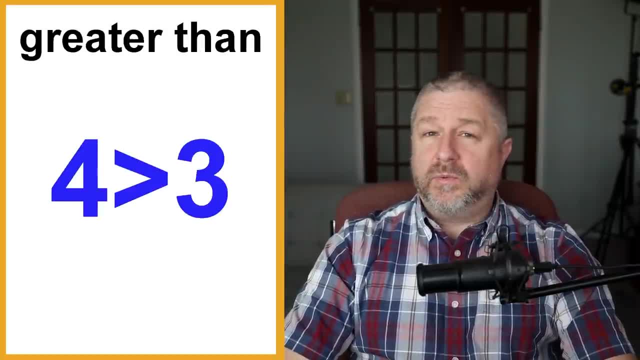 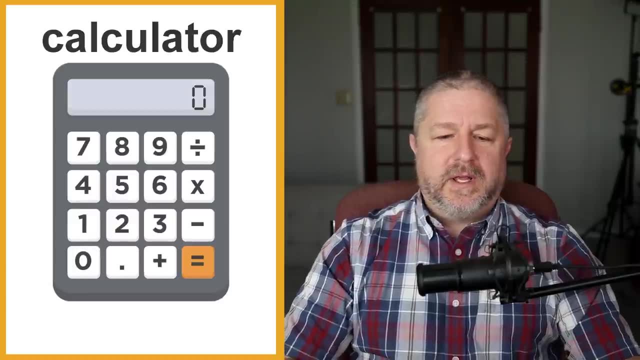 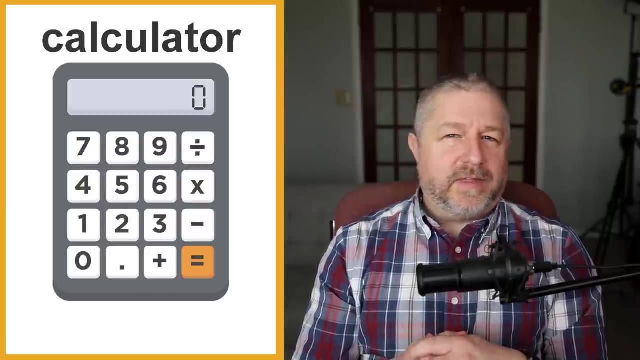 if you were to compare numbers and if you wanted to write that, you would say four is greater than three And three is less than four. So I talked about this earlier a bit, One of the cool things about the world and one of the negative things. 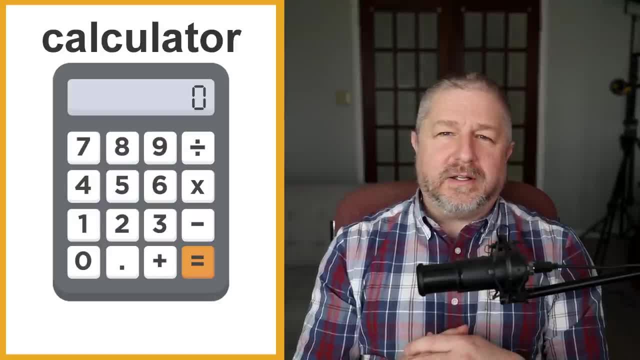 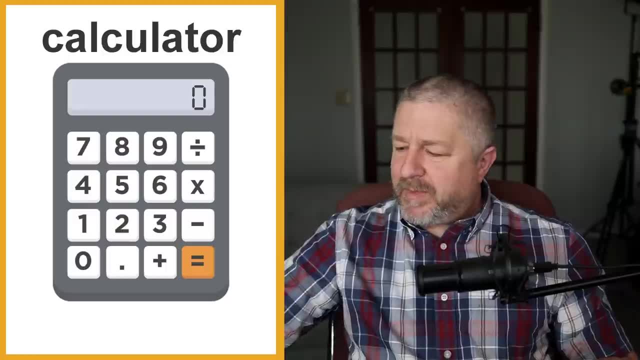 about the world is that we have calculators. So calculators are handy little devices that we can use to calculate the numbers, that we use to solve math problems Or to figure out the answer to equations. I think maybe I'm old here, but I 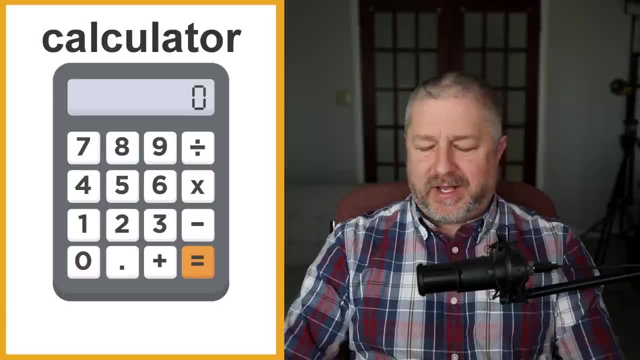 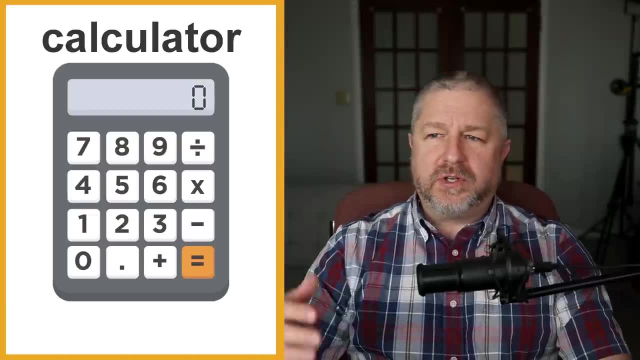 think kids use calculators way too much. I think that kids should know how to do a lot of basic arithmetic in their heads, if not all of it. You should know your times table up to 10 or 12. Like you should be able to do. like 12 times one is 12.. 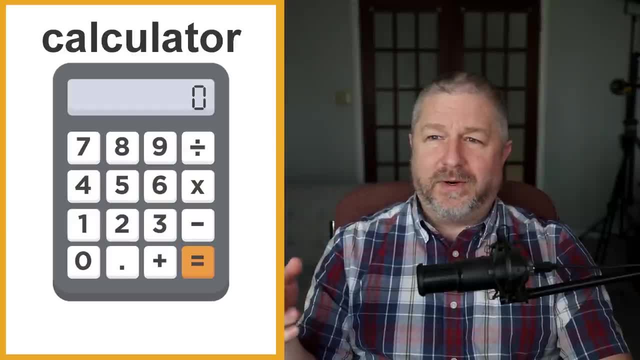 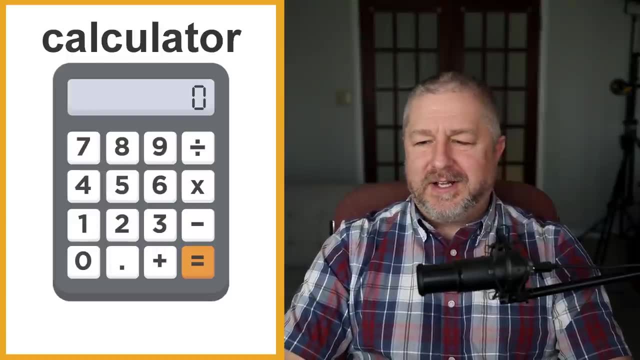 Twelve times two is twenty-four. Twelve times three is thirty-six. Four is forty-eight. I gotta stop now. I think the next answer is sixty, though, But anyways, a calculator is a handy device that will help you do math, And you might even have a 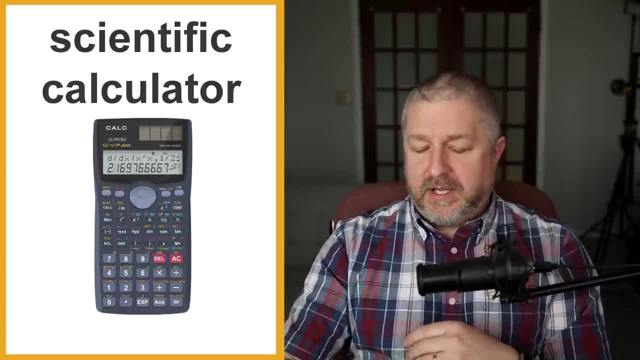 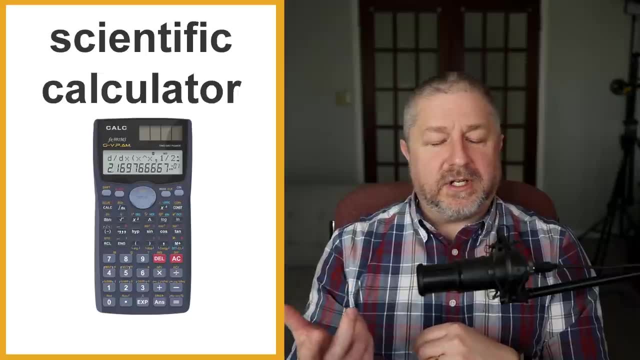 scientific calculator. I don't know all the details, but we would just call this a calculator. And when it has this many buttons, When it has sine and cosine and tangent, When it lets you do exponents and square roots, We would call this. 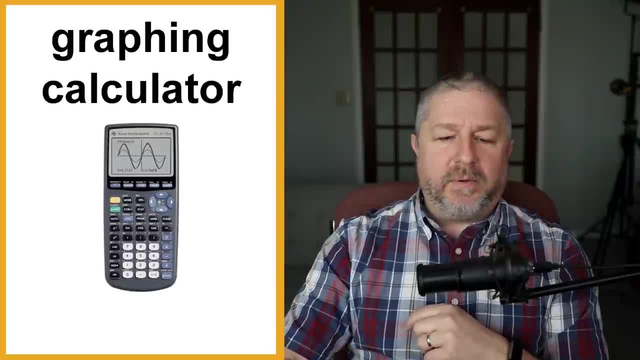 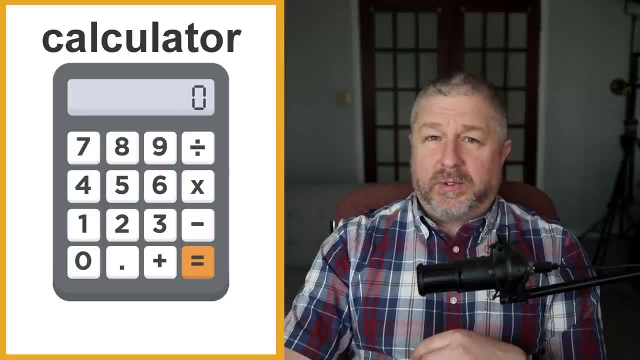 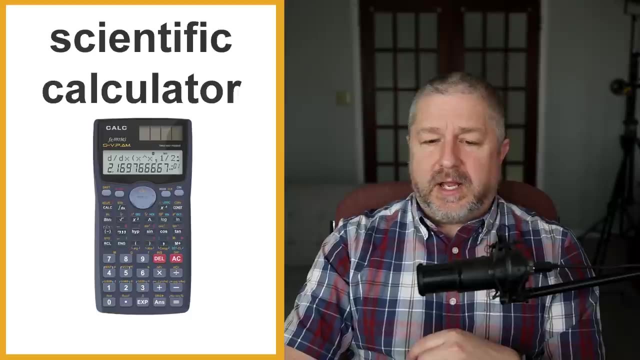 a scientific calculator And then above that we would have what you would call a graphing calculator. Generally, students don't buy a normal calculator for school. When they get to some of the upper level math, they need a scientific calculator, And when they get into the maths, where they need. 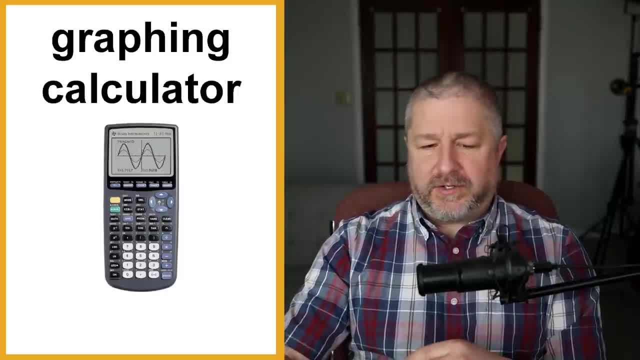 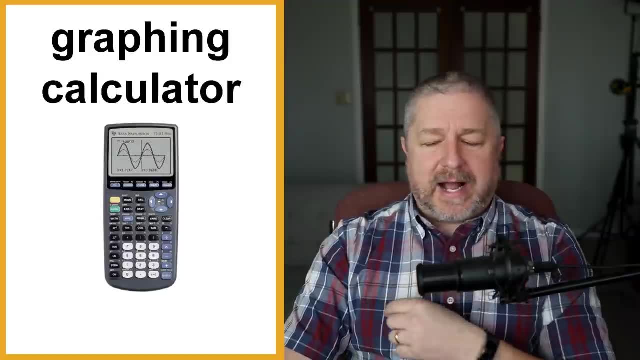 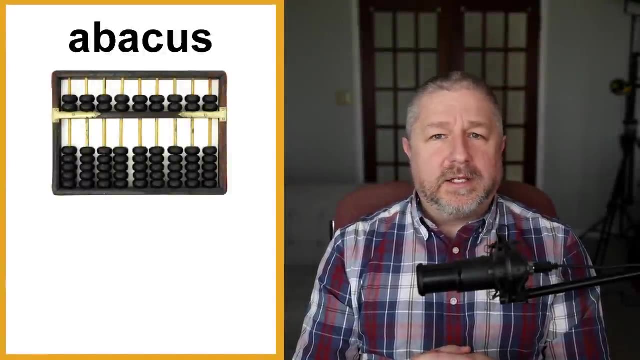 to do some graphing. they will most likely get a graphing calculator. So this is a cool calculator, because not only can you do math equations, you can actually have it graph some of those equations for you. A long time ago there was something called an abacus When I was in grade one. 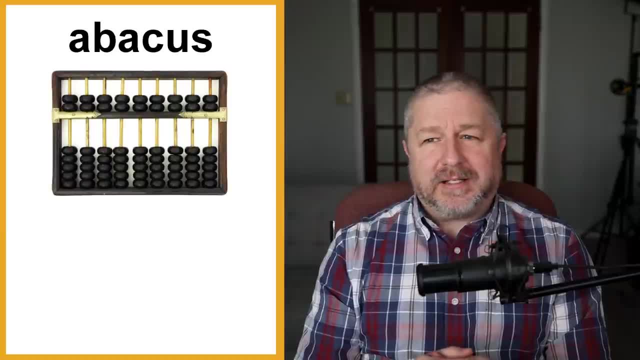 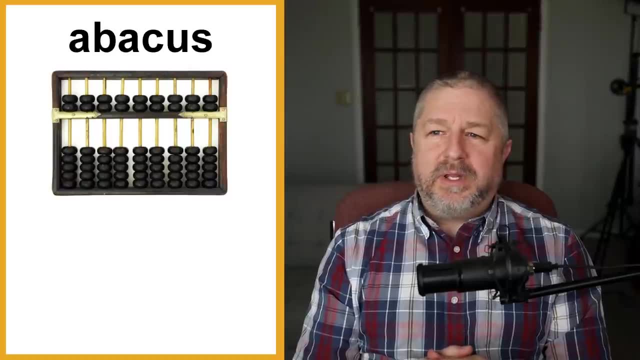 when I was like six or seven years old, there was an abacus in my classroom that we could play with and our teacher taught us how to use it. We didn't use it in math class, but we used it kind of as something we learned in history class. An abacus is: